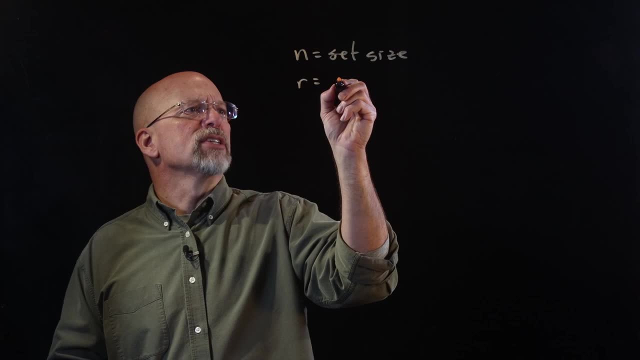 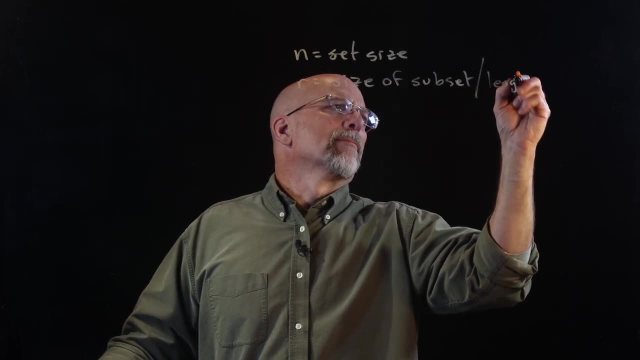 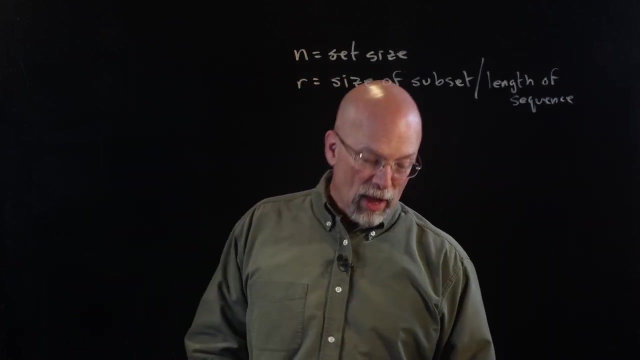 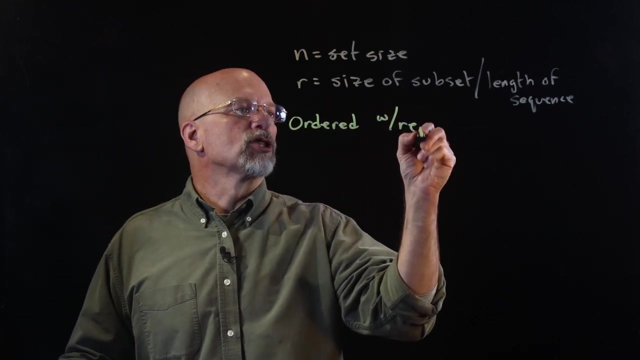 in order to create our sequence or our subset. And r is equal to the size of the subset, otherwise the length of the sequence. Now, what have we done up to this point? Well, remember, if we were to have, let's say, ordered right with repetition, Now ordered. 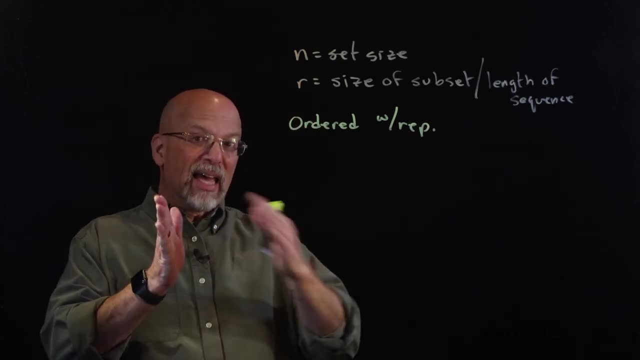 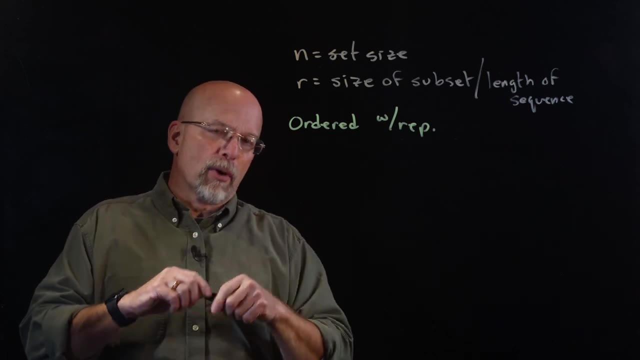 with repetition, said that I can. every time I pick an element in our series and whenever we're looking at ordered, we're talking about a sequence right? So any time we pick an element from our sequence, we've got n options to pick from, So it becomes n times, n times. 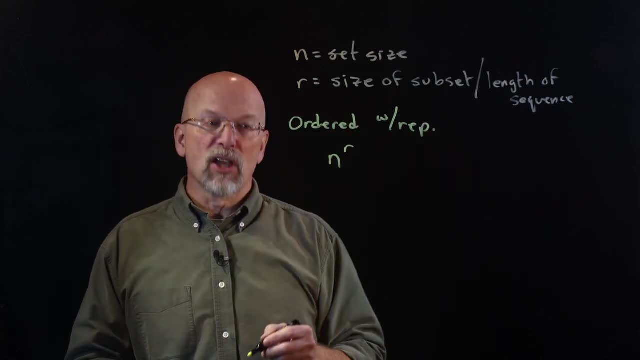 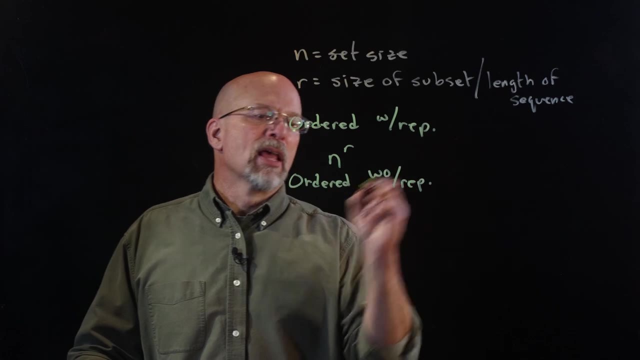 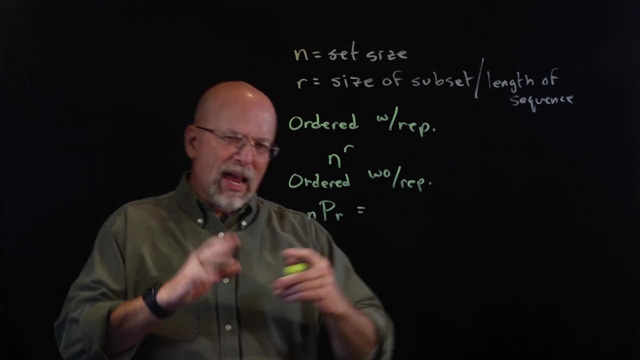 n times, n r times, and that gives us n to the r. Now, if we did ordered, but without repetition, we had this thing, npr. these permutations, And there was an expression that we had for this. And, if you think about it, if we had 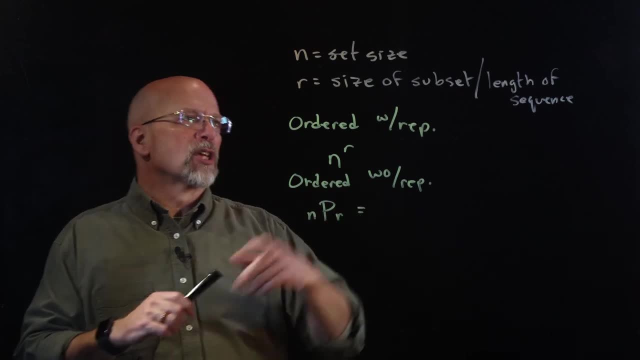 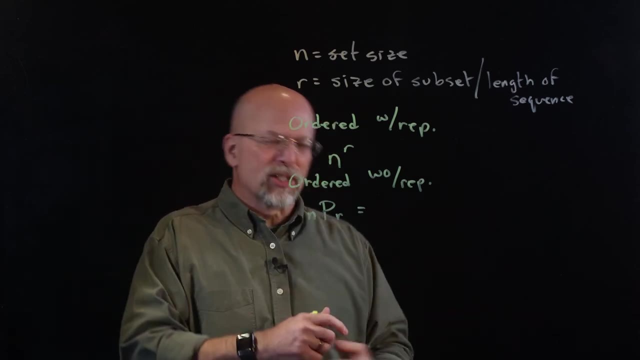 a full sequence. if we just basically were going to order our sequence from all n elements, we'd have n to choose from for the first digit, n minus 1 to choose from, for the second digit, n minus 2 to choose from, and so forth. That ends up being n factorial, But not all sequence. 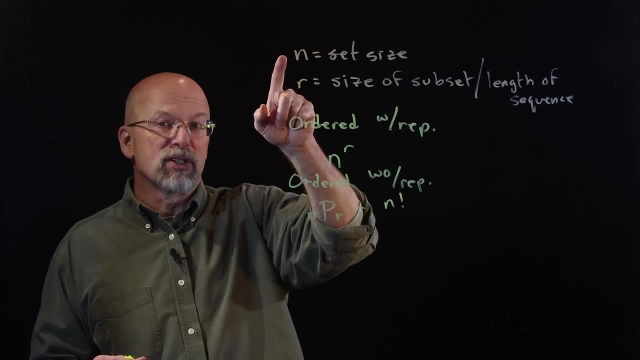 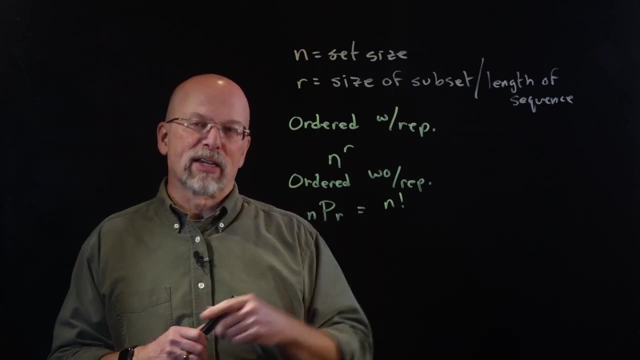 is are going to be pulled from a. not all sequences that are pulled from this set size of n are going to be of length n. And remember we also talked about how n minus 1 also did the same. you know n factorial solution. But if we have a sequence that is at least 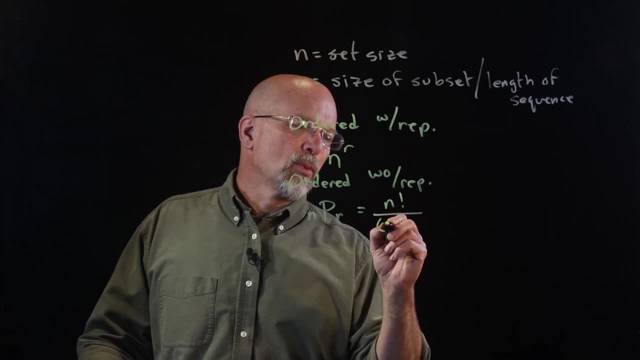 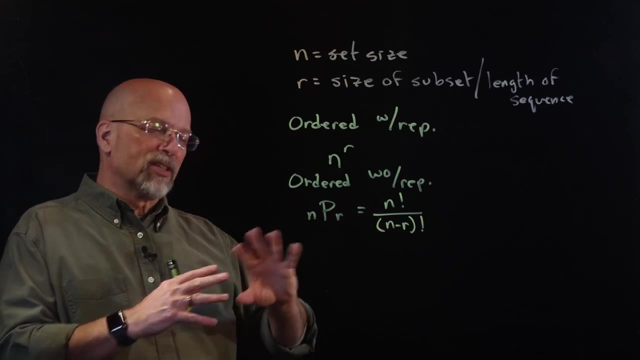 two shorter than the number of elements in our set size. then we divide by n minus r in order to pull out all the options that were left over, in order to give us every possible sequence from the elements that were not left, that were not pulled from, And so 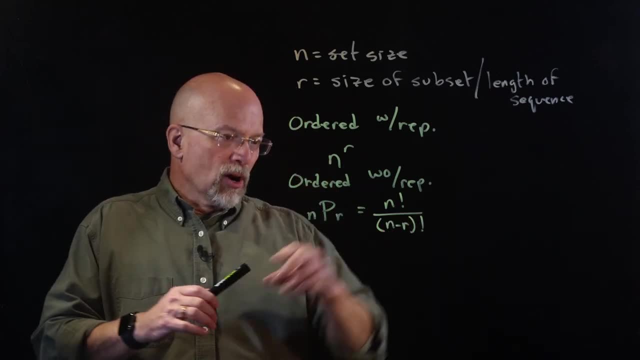 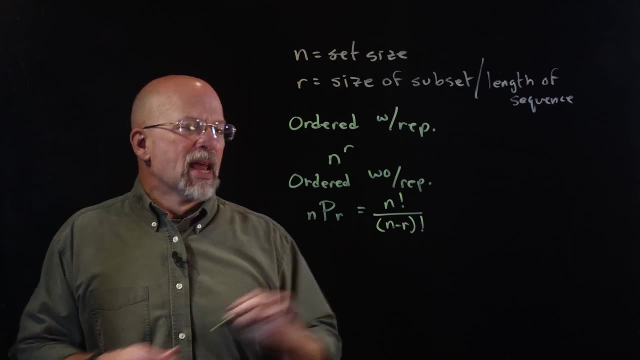 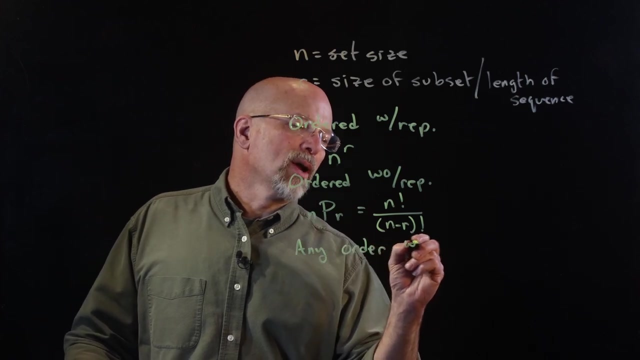 we're not picked for the first r elements, So there are our first two. you know permutations and sometimes you'll see this exponentiation or multiplication principle. Now any order. we started with with the last lesson, So we have any order, but without repetitions. 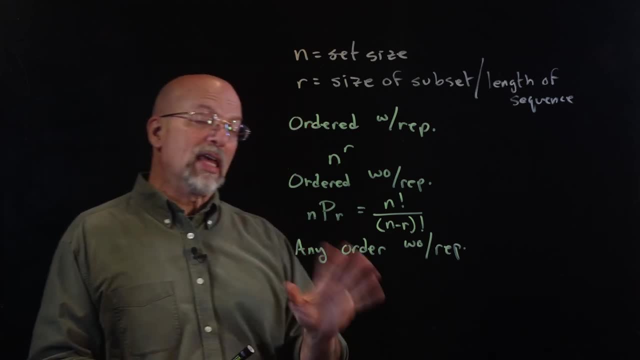 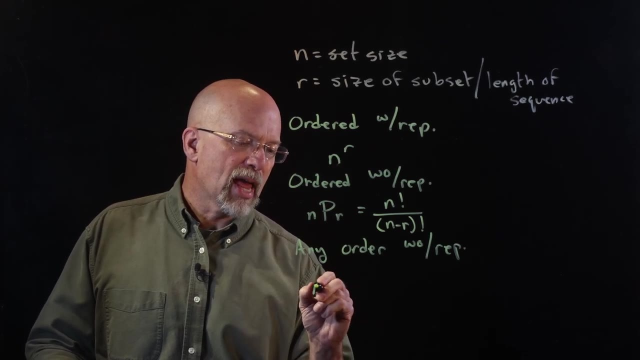 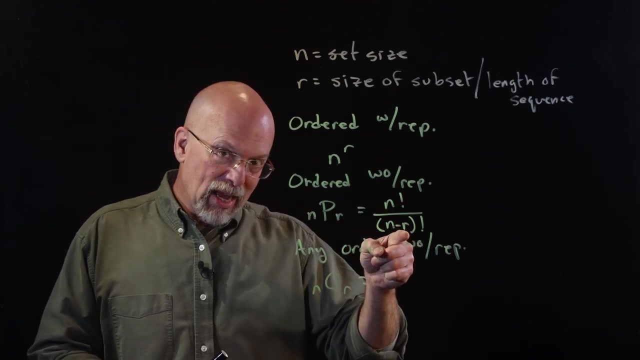 Remember, we're going to do any order with repetitions for this one. Now, any order without repetition is also referred to as combinations, And so you had this expression: n, square, n, c, r- And what you did was you took the permutations and then from the r elements 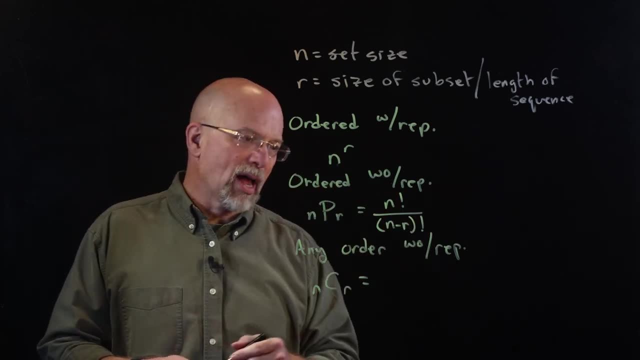 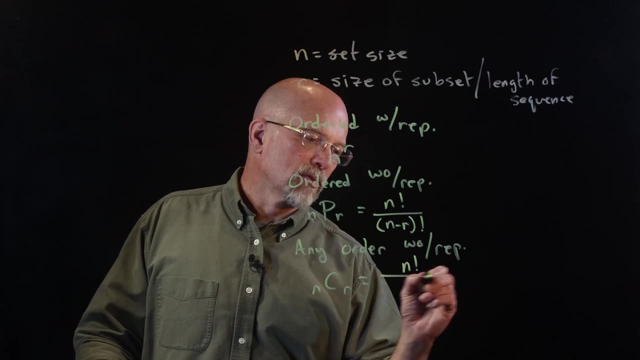 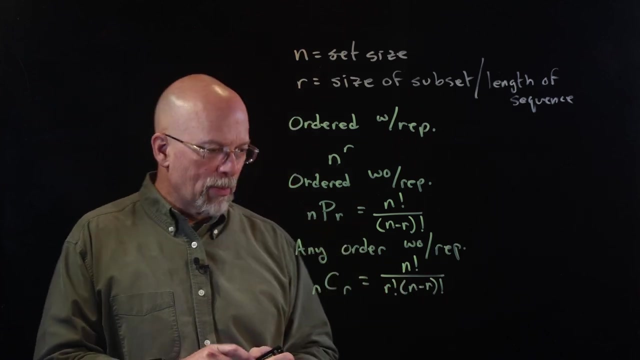 you divided out any possible ordering you could have for those r elements And that would give us the total number of any order combinations. So that gave us n factorial divided by n minus r factorial, just like the permutations. But then we also divided. 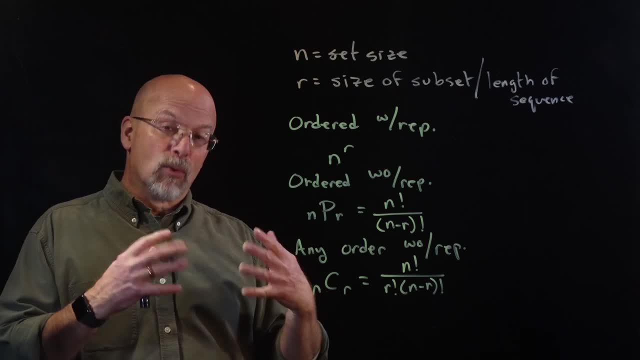 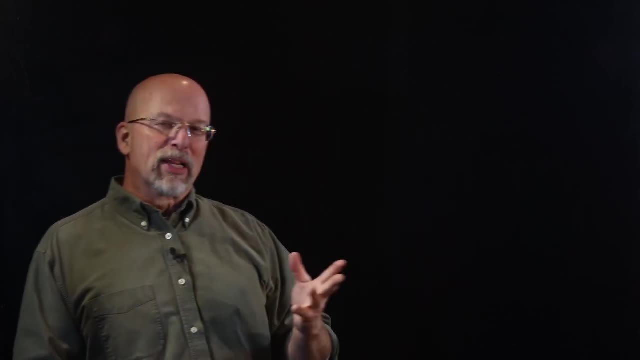 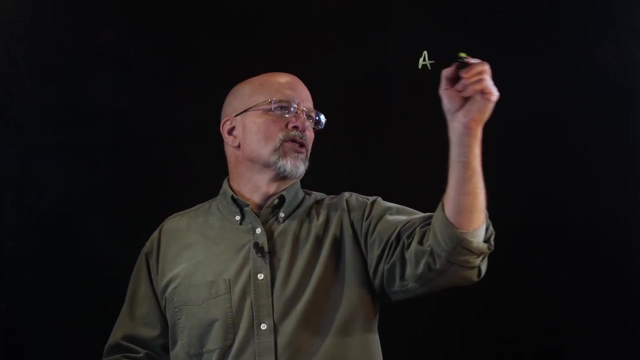 by r factorial in order to make it so that they didn't have to rely on any sort of an order. Now let's assume that I have three coins. I'm just going to throw them out on the table and they're going to come up with some combination of heads and tails, And maybe my coins will. 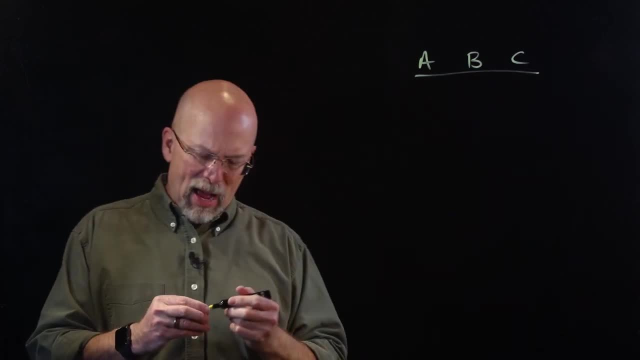 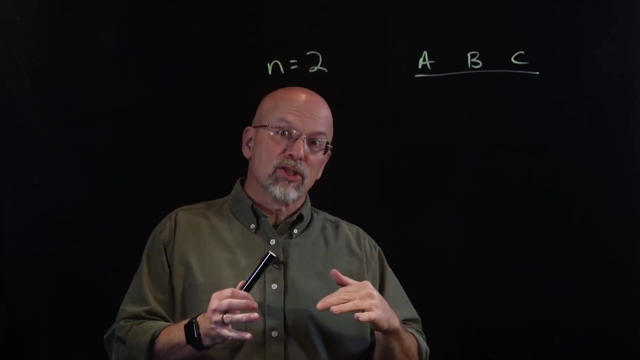 just say a, b and c. There are how many possible ways that they could come up. Well, n, our set is actually equal to two. It's either heads or it's tails. So the set we're pulling from is either heads or tails. Now, since we can have repetitions, I can actually have 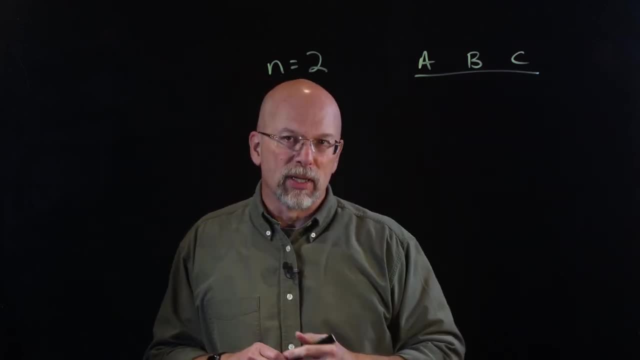 more than one set of heads and tails. So I can actually have more than one set of heads or tails. So I can actually have more than two different elements in the sequence that I'm putting together. Now, how many times am I going to be picking from this set of 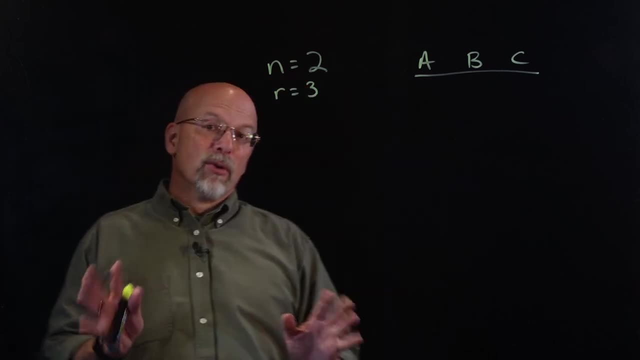 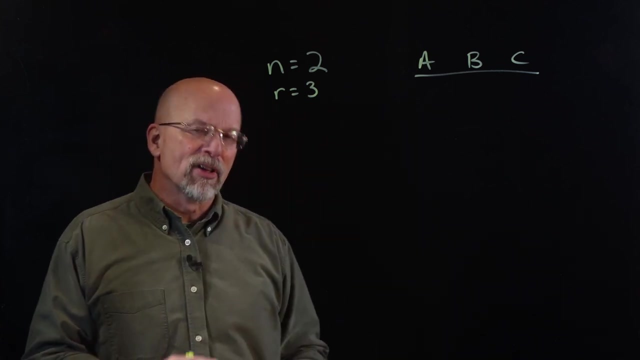 two. Well, r is going to be equal to three. Now, if you remember, whenever we figured out combinations, we started out by saying: how many possible permutations do we have? And then can we pull out order by dividing by our fact territorial in order to make it. 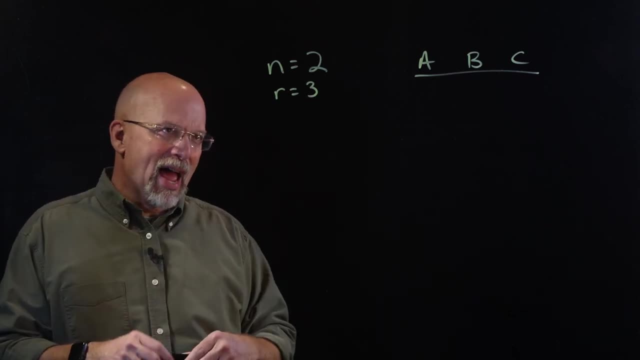 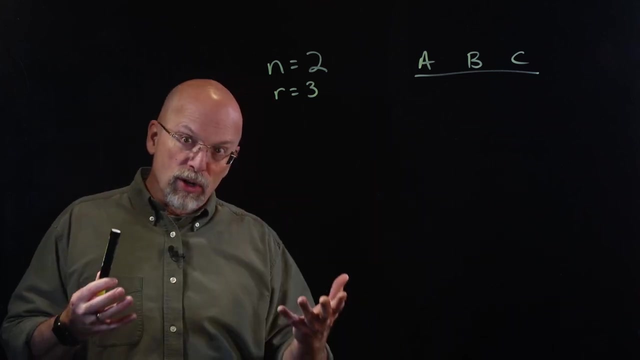 so that any of the manifested orders could be divided out. Let's see if the same thing works for this. You know, any combination or, excuse me, if we have an order, a specific order, but we can repeat. then we had that n to the r, So two to the three. 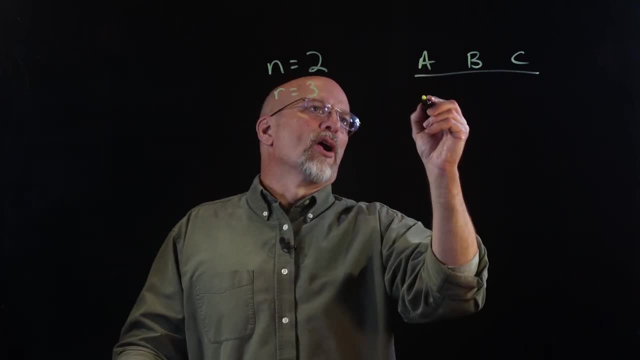 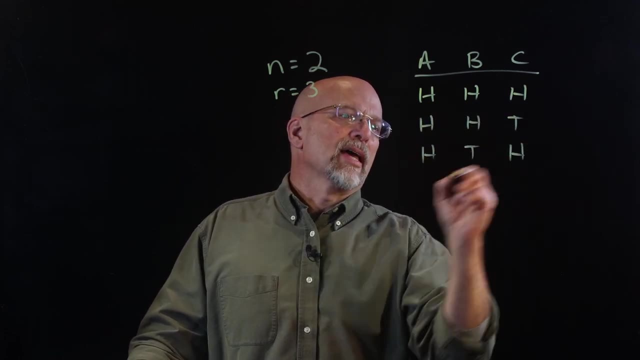 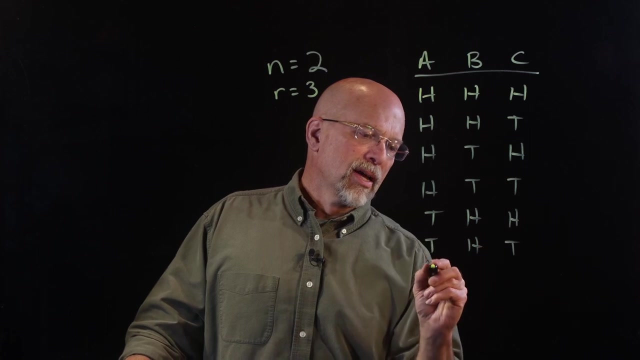 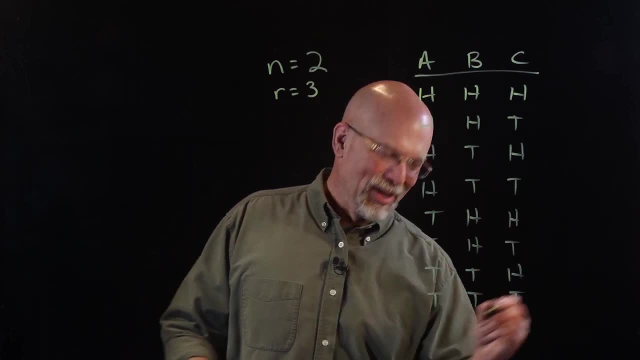 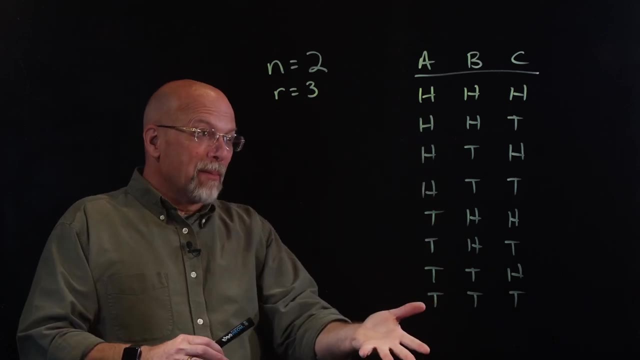 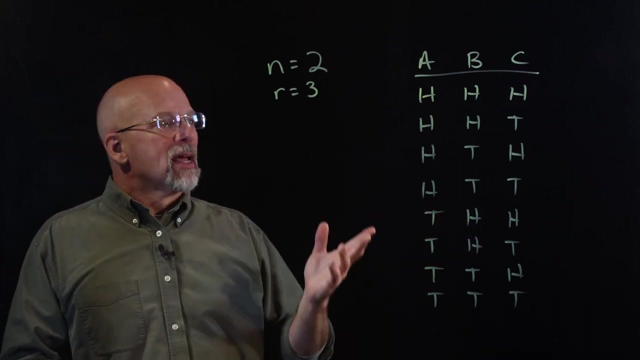 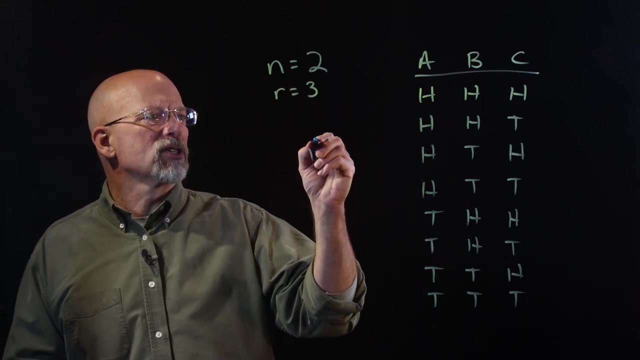 tails, tails, heads, and tails, tails, tails. well, is that all of them? I hope so. so the idea is there is every possible combination or in order in an ordered set with order with repetitions allowed right. so I should be able to just divide out the ways these can be ordered right, and so it should be something like n to. 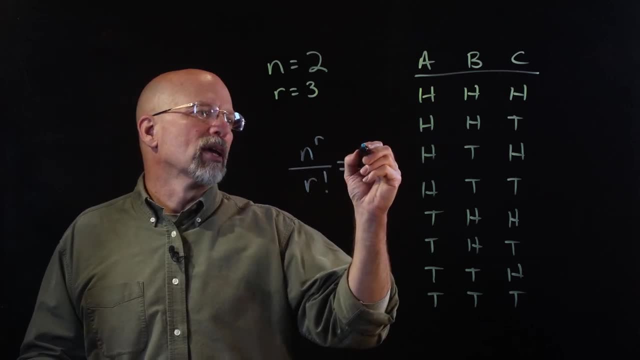 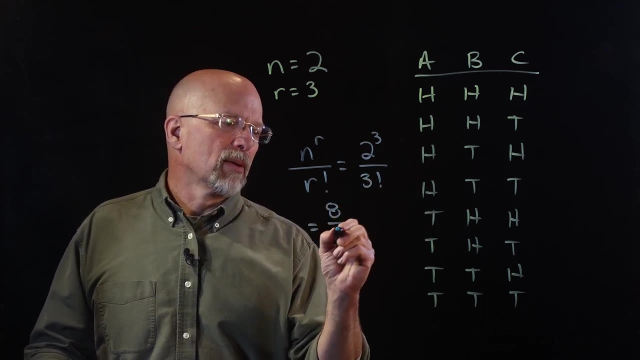 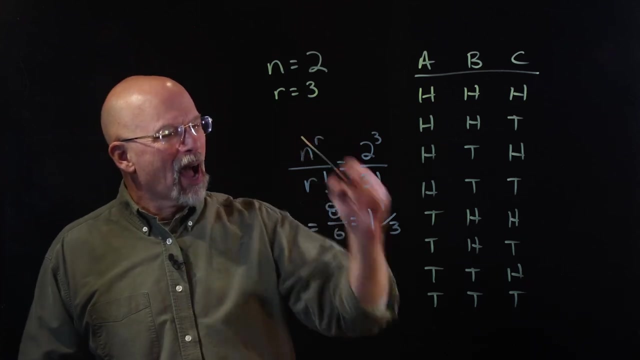 the R divided by R, factorial, which would give us 2, to the 3 divided by- and what do I have? 3 factorial that would give us 8 divided by 6, which gives us 1 and a third. don't think that's going to work. this is not an option. this will not work. 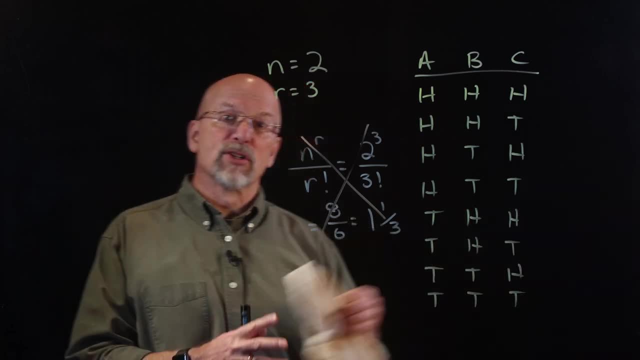 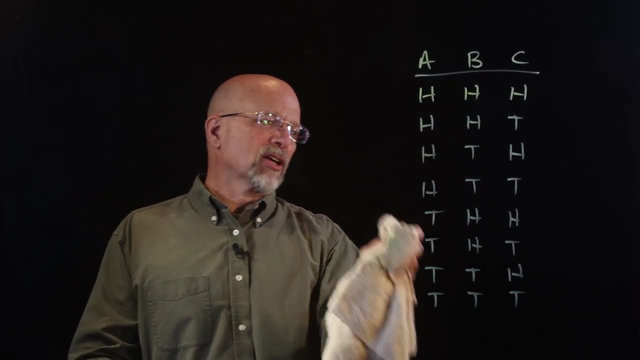 for us, so we've got to come up with some other way to represent these combinations. now, what number are we looking for? what target number are we looking for? well, let's take a look at our list and see what our duplicates. okay, the heads, heads, heads, that one. 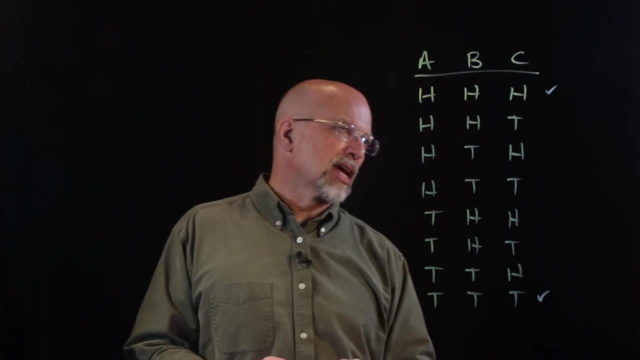 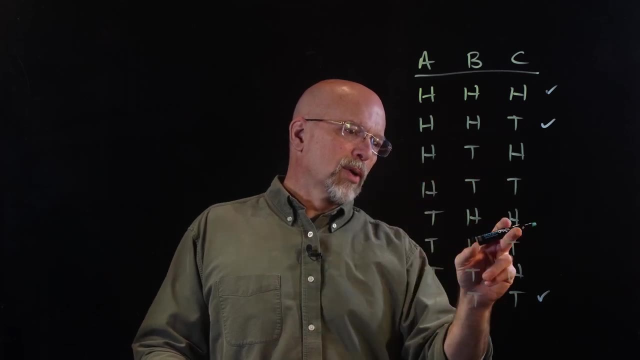 there's no other one that's a: heads, heads, heads, just like tails, tails, tails. there's no tails, tails, tails. here's two heads and a tail, where else is another two. there's two heads and a tail, so that one can't be used. this one says two. 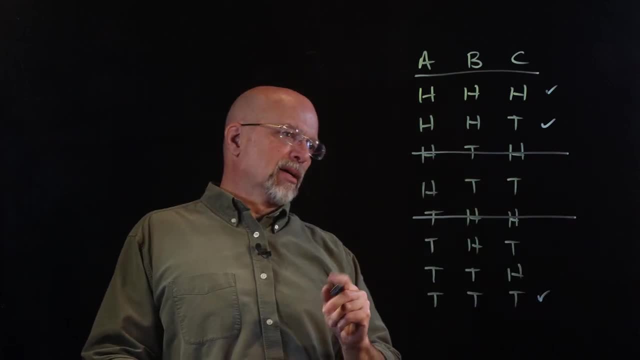 heads and a tail that can't be used. is there any other one? I don't see one. now here's two tails and a head, so we need to count that one, but we need to cross out any other heads and tails that can't be used. now here's two tails and a head, so we need to count that one, but we need to cross out any. 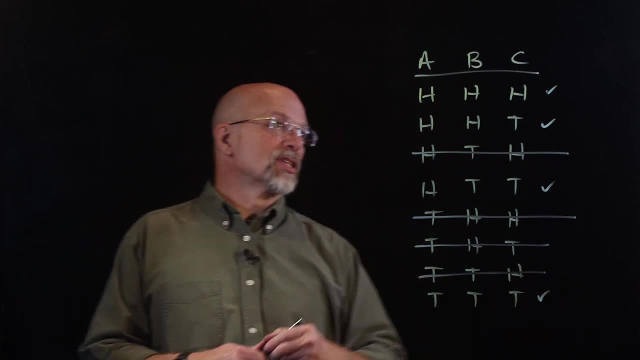 any other heads and tails that can't be used. now here's two tails and a head, so we need to count that one, but we need to cross out any other two tails and the heads, So what we're looking for is actually an answer of four. Now, 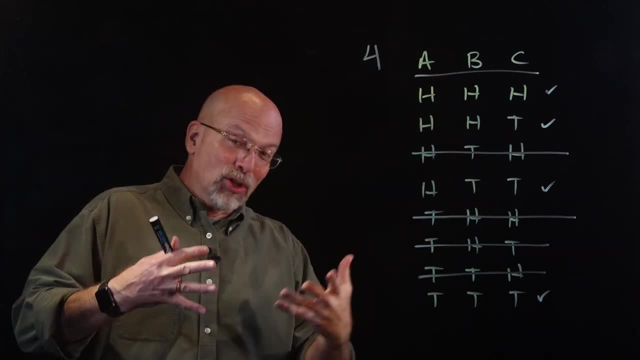 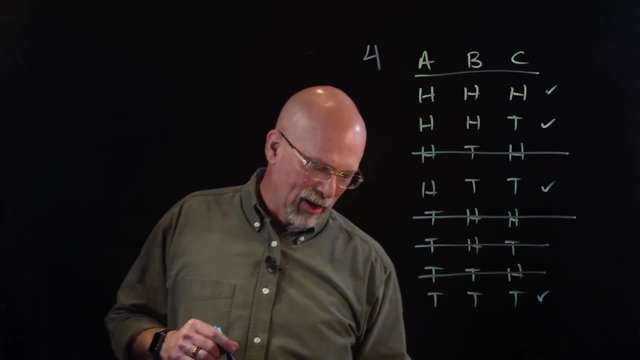 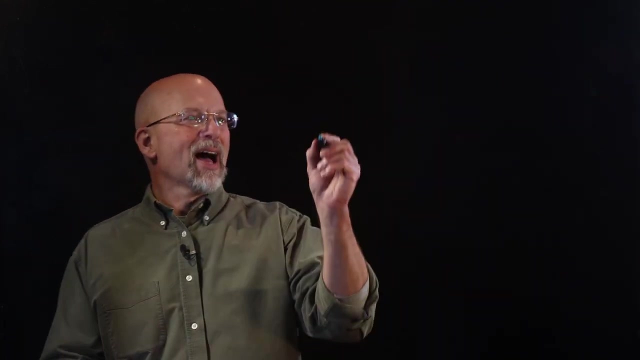 I'm not saying that this is a proof as to how the solution we come up with, if it works, if we simply apply it to this and get four, but I'm just showing you. the target number that we're looking for here is four, So let's try modeling this. I am going to make a bucket to hold the tails and a bucket. 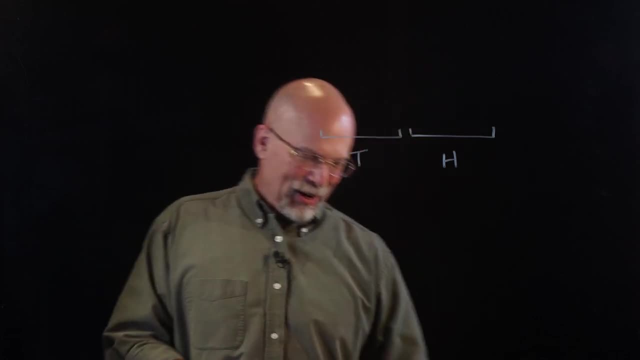 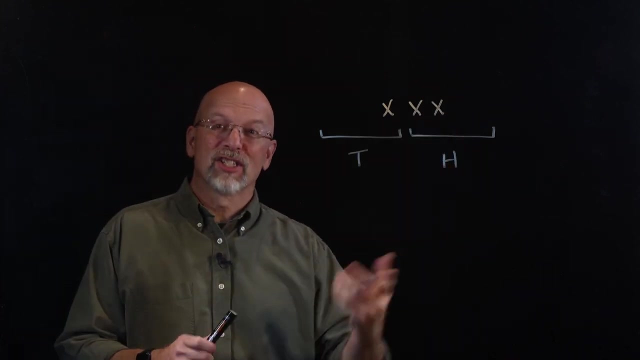 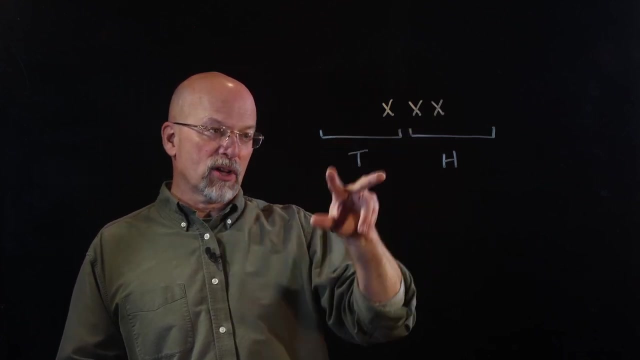 to hold the heads. Just go with me here and let's say that I've got my three rolls, all right, or my three tosses of the coin. Now, if you see these three tosses of the coin, I could move them all the way over here so that all three tosses are tails, or I could move them all the way over here. 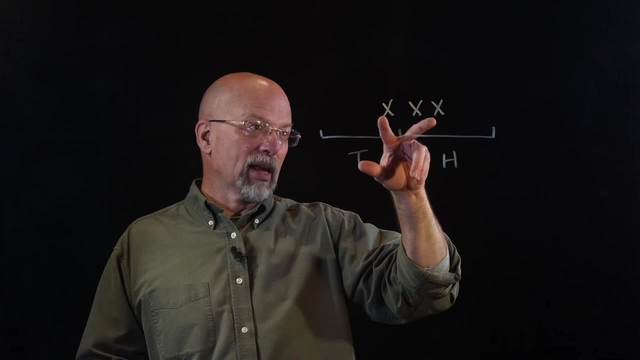 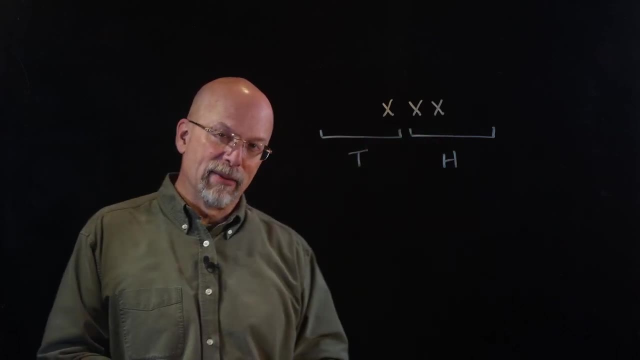 so that all three tosses are heads. or I could have it somewhere in the middle, like here, which is one tail, two heads, or I could move it over one position this way and have two tails and one head. Now, another way of representing this or modeling this would be to say: I've got 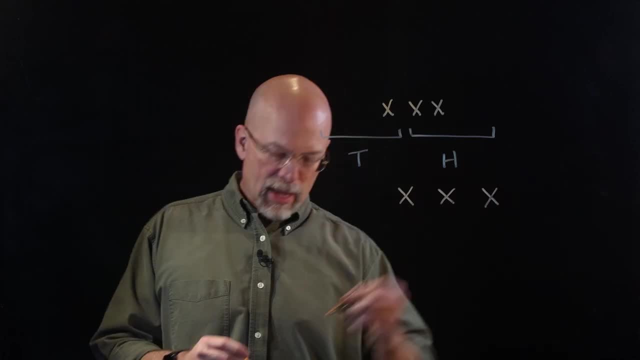 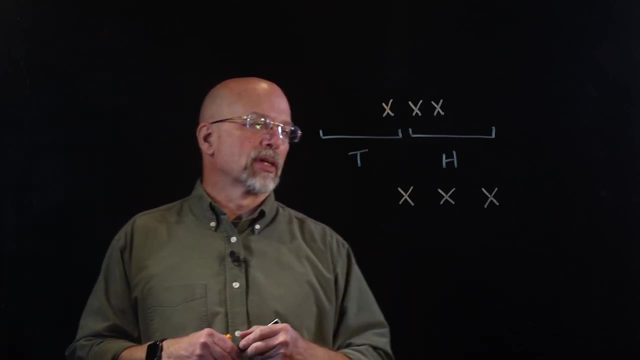 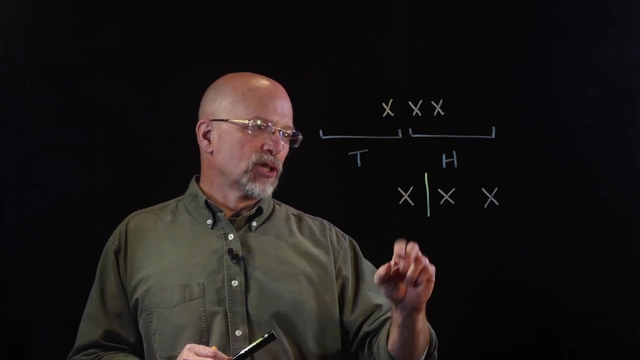 the three tosses, all right. and then a divider, some sort of a divider that separates which group it's going into. Is it going into the tails group? Is it going into the heads group? So right now it would look like that, all right, So I've got one tails and two heads. If I moved this so that it. 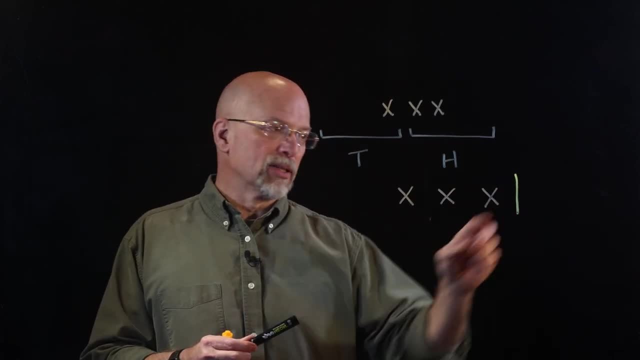 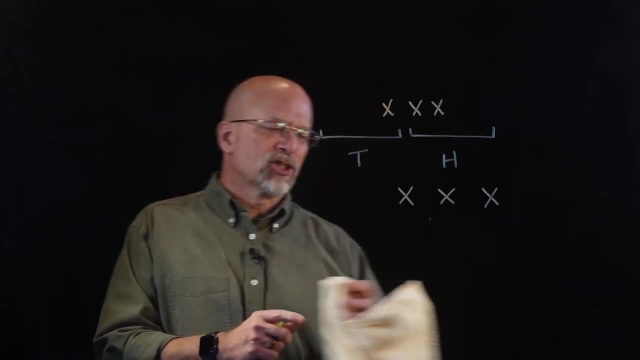 was over here, I would have three tails and two heads. So I've got three tails and two heads, Three tails, no heads. So this divider basically shows me where the partition is between our heads and our tails. Let's try drawing this a slightly different way and one way, a way that will give us. 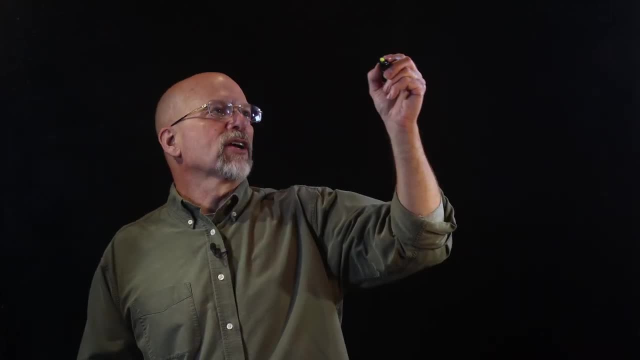 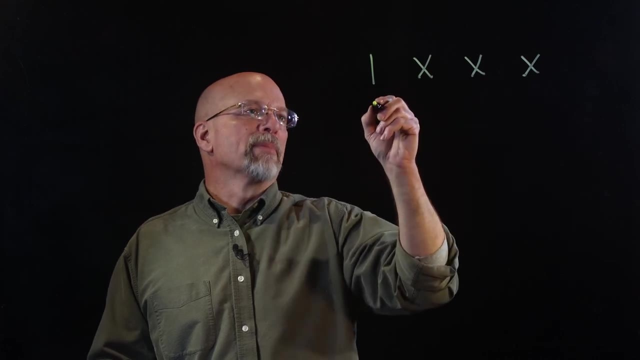 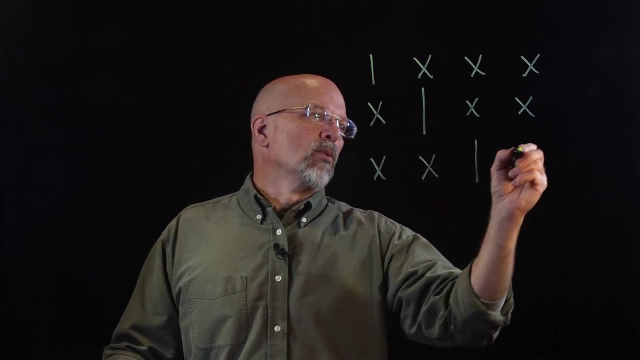 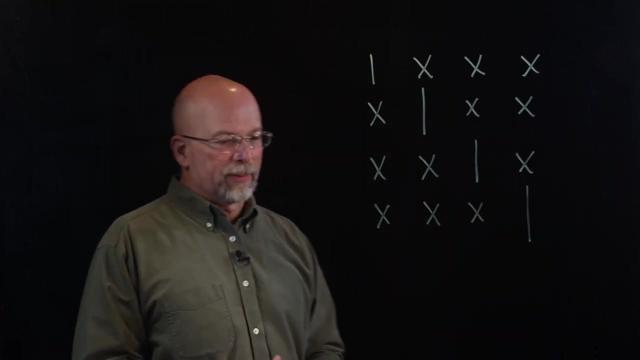 the ability to model all four options. So I could have the divider and then x, x, x I could have, and that would be three heads, right? I could have a tail and two heads, I could have two tail and one head, or I could have three tails and no heads, And those are all of our options, right? 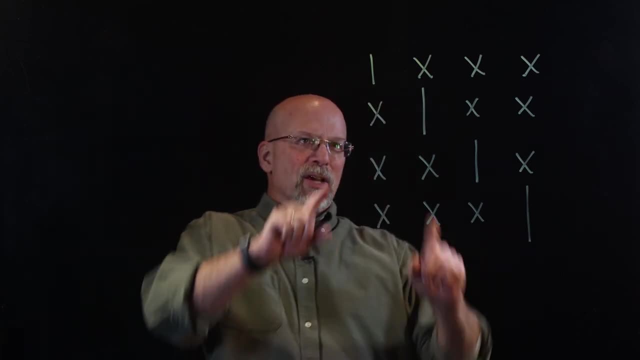 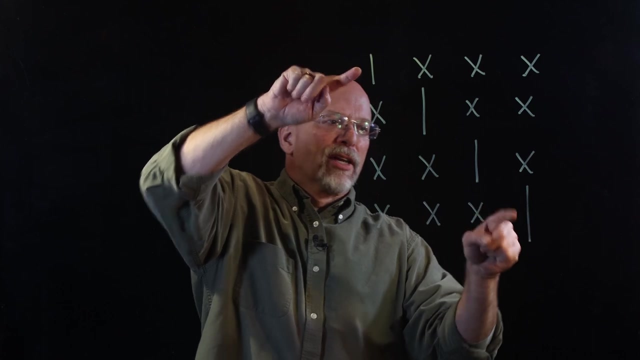 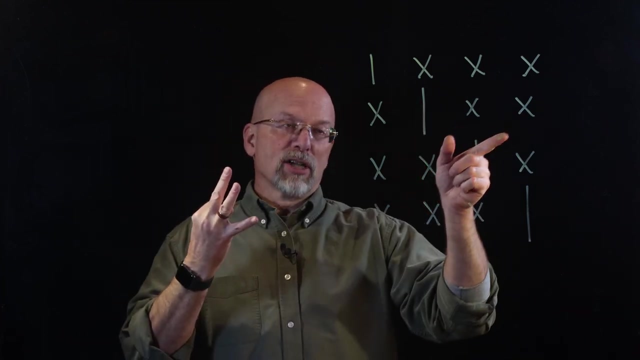 Well, what is this actually? If you look at this, a picture picture a slightly different way of viewing this diagram here. Picture this divider as being an empty slot out of four slots. So I have three options. Those three options are my tosses and I have four places where I could put. 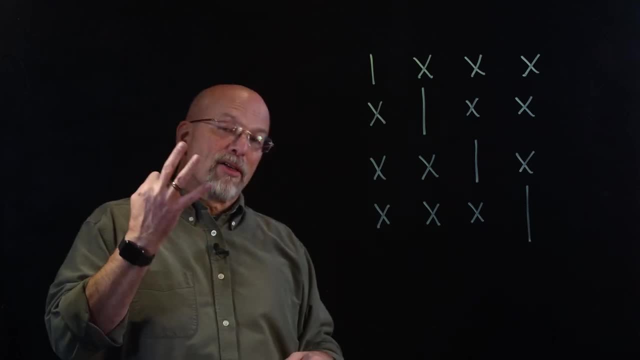 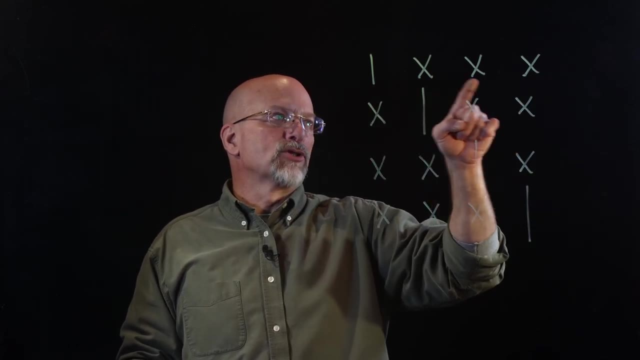 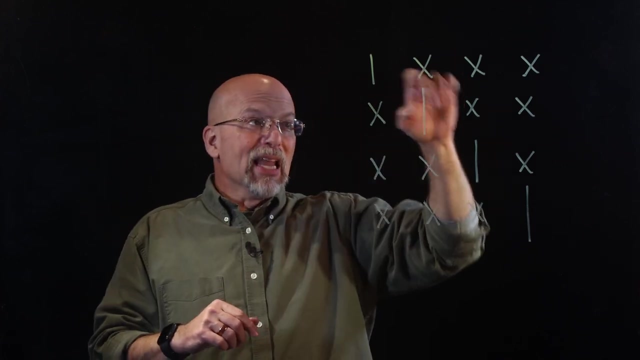 these options. Excuse me, I'm going to try that again. I've got three items to place and four places to put it, So I've got four slots and I just so happened to put the three items, or three elements, in these last three slots. Only one element can hit each one of those slots: Four places. 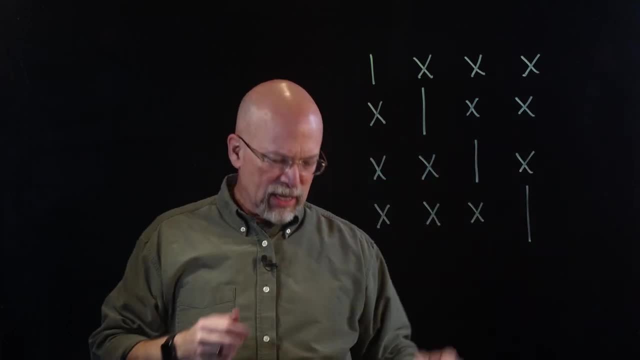 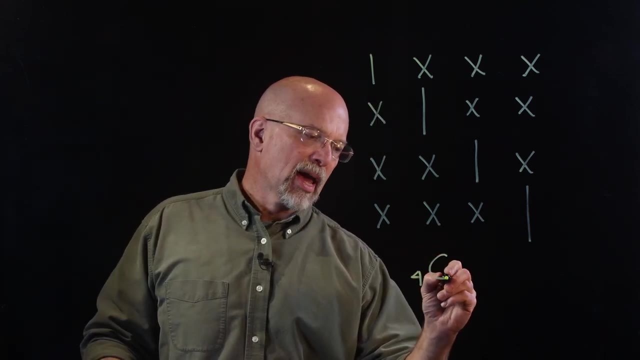 to put something. Three somethings to put. How many different ways can I do that? Well, that sounds an lot like. I have four places to put something and I'm choosing three. the order in which I choose them doesn't matter, I don't, I could pick this one. 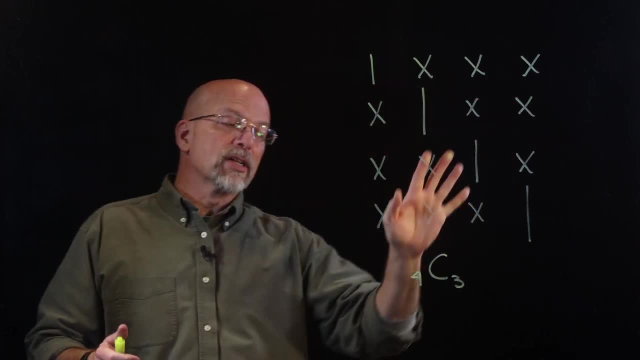 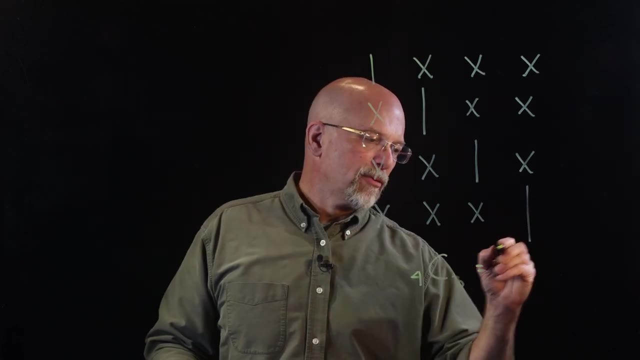 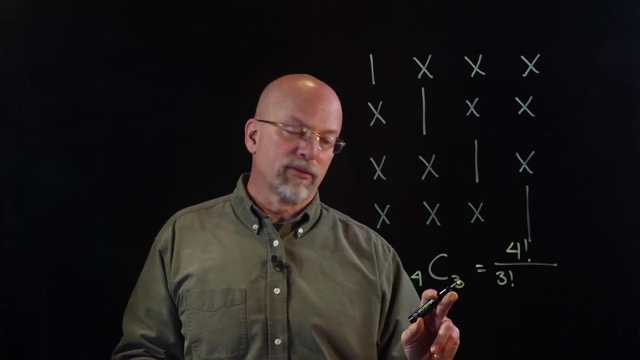 first, then this one and this one, or this one, this one, this one, the order doesn't matter. I've got four places to put something and three somethings to put. so this ends up being what: four factorial right divided by well, three factorial is the number of- is R right, and then four minus three factorial. so this becomes: 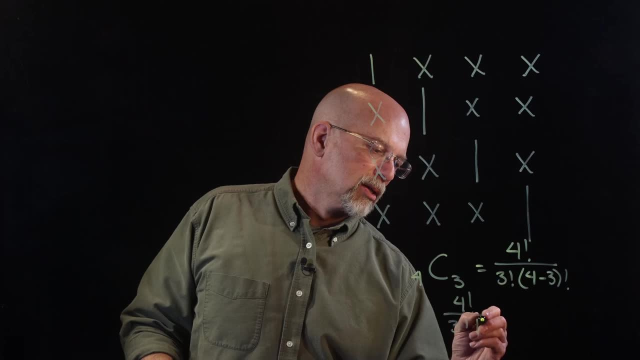 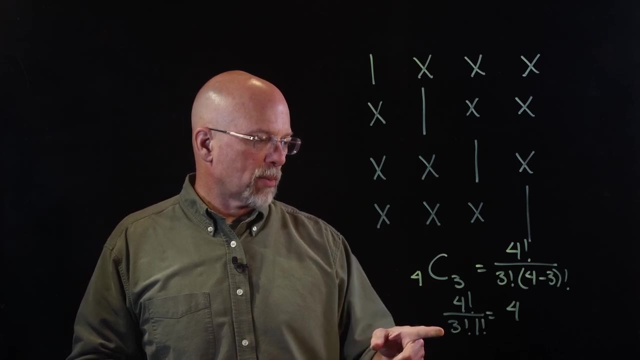 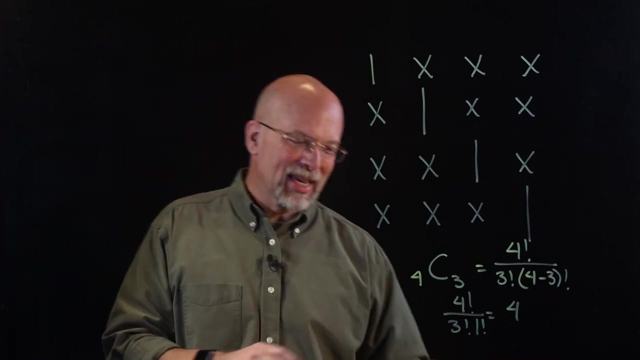 four factorial divided by three factorial times one factorial which is equal to four. so this is four times three times two times one. divided by three times two times one times one, that's just equal to four. that is our answer. now let's talk about this in a little bit more. I don't know mathematical way. 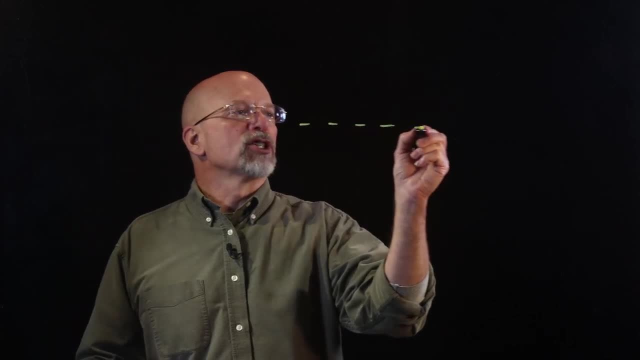 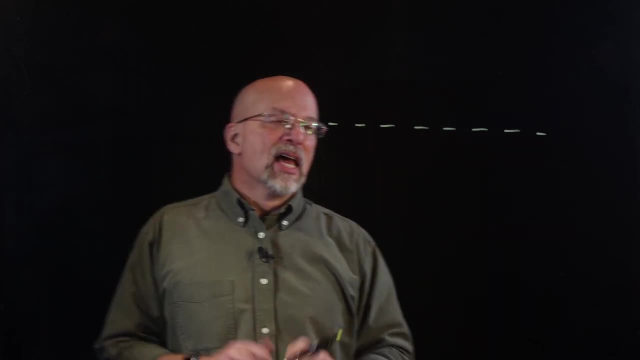 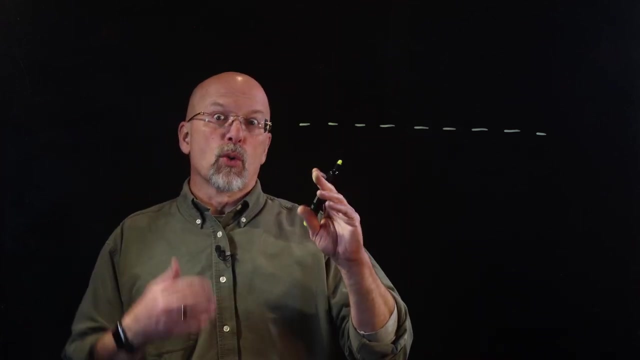 so what I'm looking at is I've got a bunch of spaces to put elements, so in this case, I've got one, two, three, four, five, six, seven, eight, nine. this would be our tosses, our coin tosses, and then what I need is to have dividers or spaces. 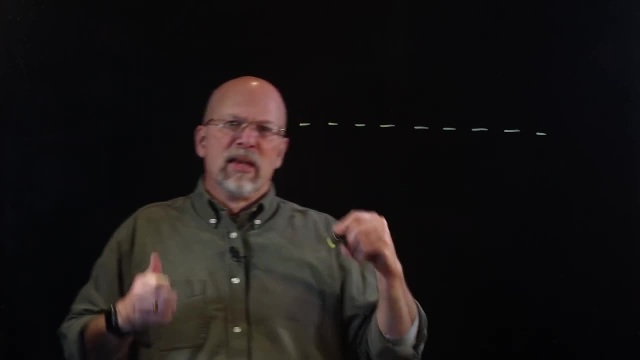 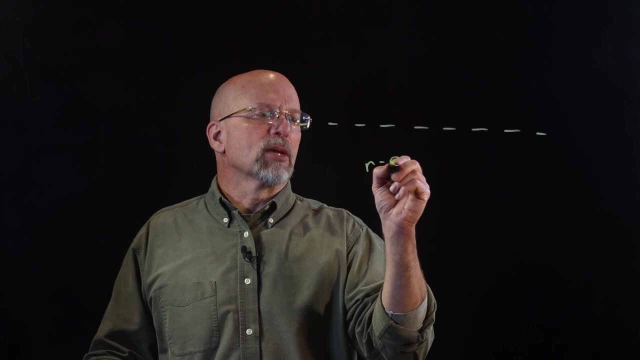 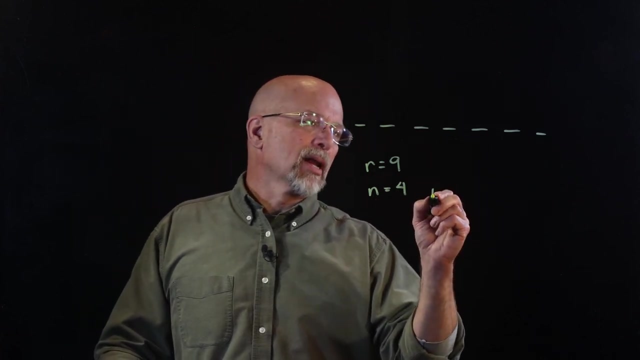 that are going to divide these up. so let's say, let's just so. so I've got one, two, three, four, five, six, seven, eight, nine. so what I've got is R is equal to nine, nine, nine, nine. and let's say n is equal to four. well, any equal to four means that I'm gonna. 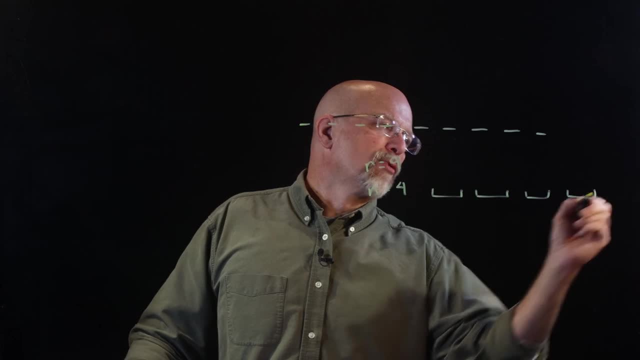 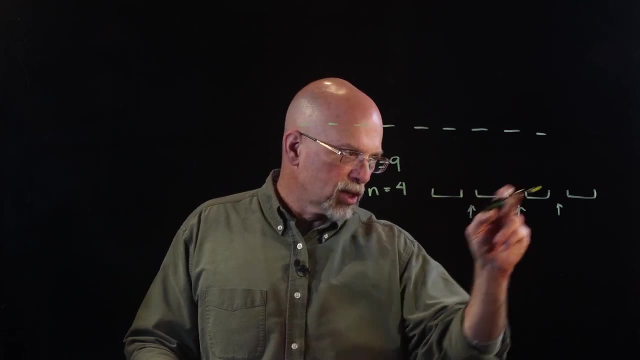 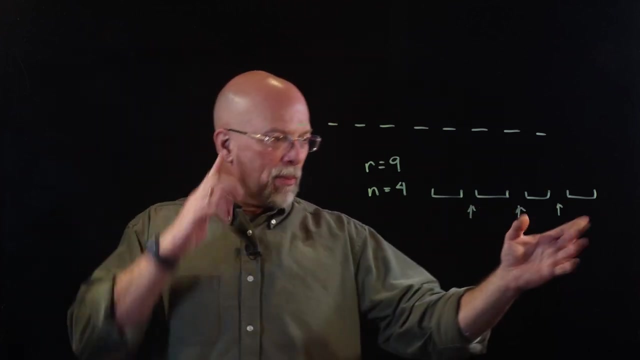 have things grouped together in four spaces and in between each the of these spaces, so I'll have all like items here, all like items here, all like items here and all like items here. let's just pick colors. okay, let's say it's red, green, blue, purple. all right, all my reds are gonna be on this side, separated by a. 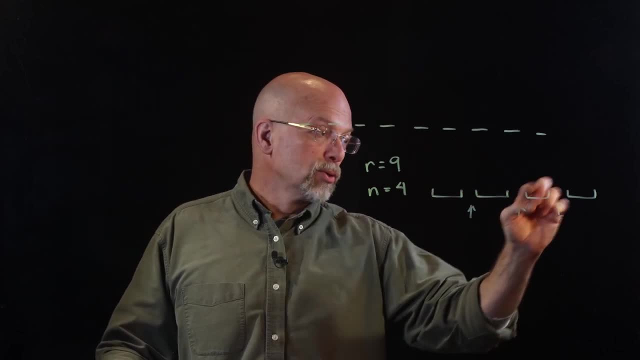 divider, and then I'm gonna have all my greens, and then I'm gonna have all my blues, and then I'm gonna have all my greens, and then I'm gonna have all my and I'm gonna have all my purples. each one of them is separated by some sort of 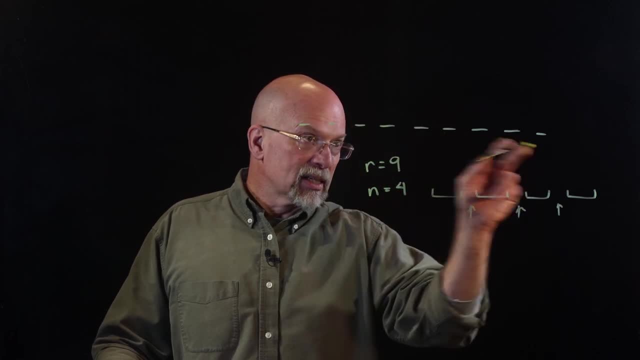 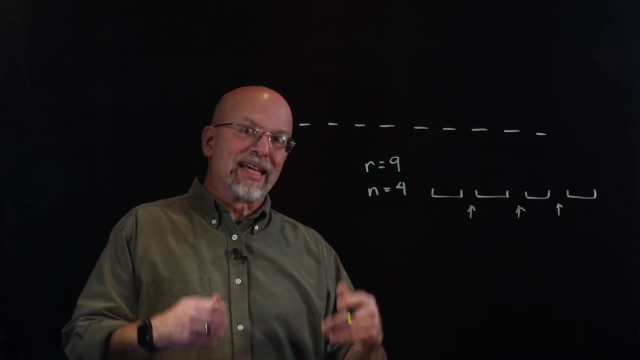 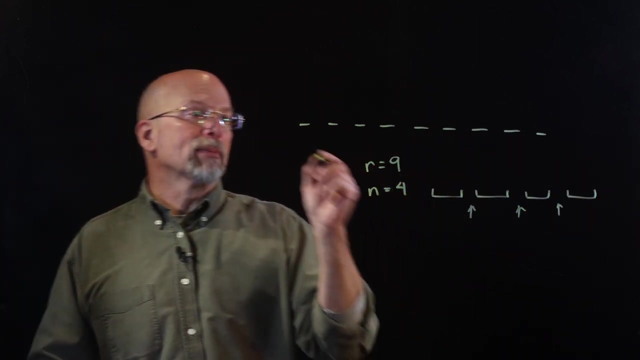 a divider, and these are where these, these spaces, these little slots, are going to be filled up. now, each one of these is going to manifest itself as an empty spot in our selected rows. so I've got what? one, two, three empty spots. so I'm gonna add one, two, three here, and so, remember, I had nine, so I could go one. 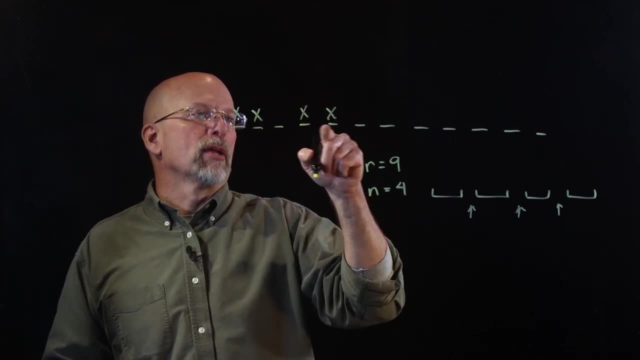 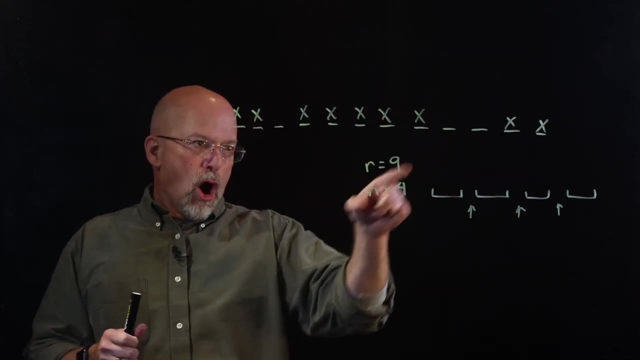 two space, one, two, three, and then I'm gonna add one, two, three here, and so I'm gonna add one two space, one, two, three here. and so two spaces: one, two, three and here. so these X's are very similar to this space. space is seven, so these X's reached from an F and an E, so what you're gonna do is: 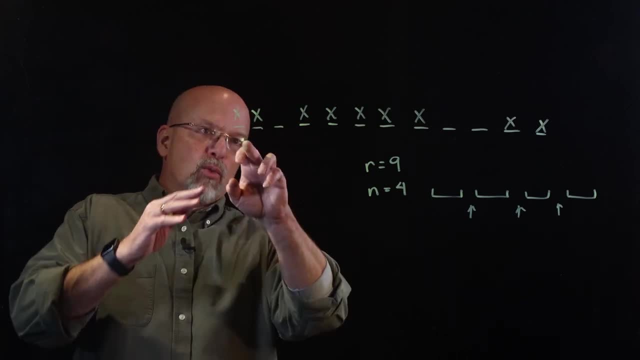 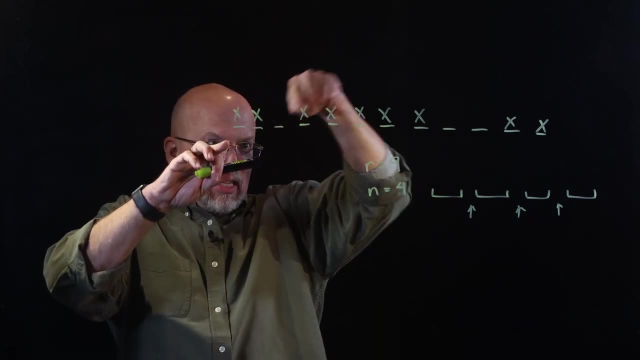 you're going to, we're going to be able to really engage each one of these spaces, and with that I'm going to grab my three. just run all of those again through your assigned space: three, four, five, six, seven, no blues, and then two barks and then to the second space. I'm gonna have nals S right: six, seven and 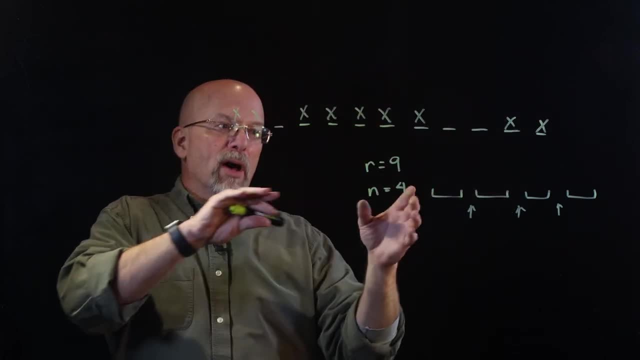 I'm going to answer to path good, I'm going to have n know m no, x equal to n. good is three, four, five, six, seven, space, space, eight, nine, so r is nine. I'm picking, pick, pick, pick ones that are of the same type. I'm going to group together and separate from the 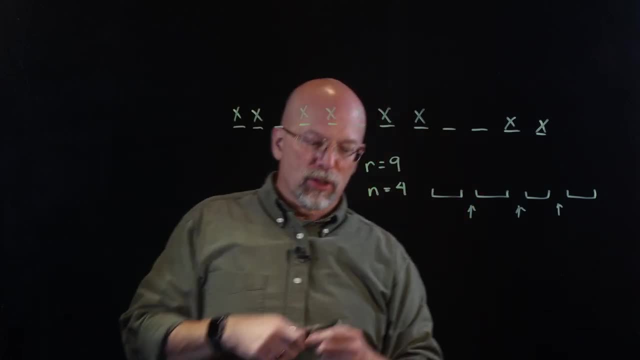 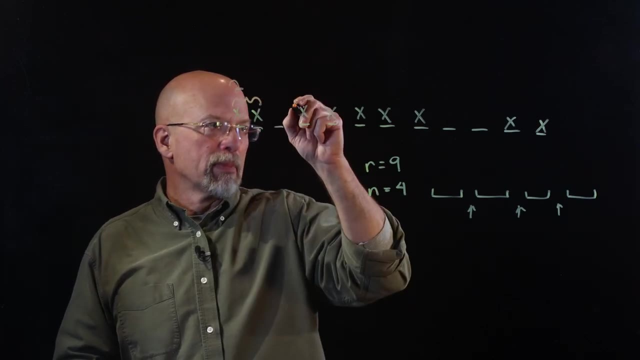 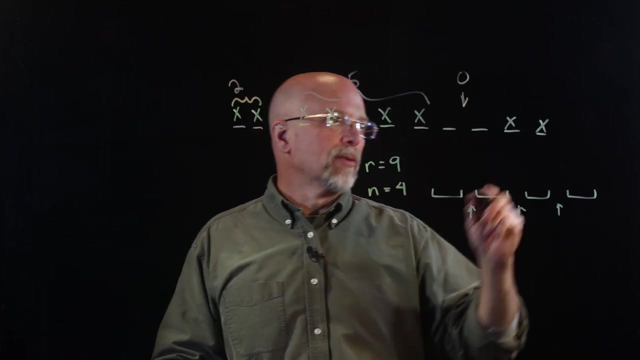 next type with a space and then separate from the next type with a space. and if you look at my patterns here, I've got two from the first element of M, I've got five from the next element of N, I've got zero from the third element of N and 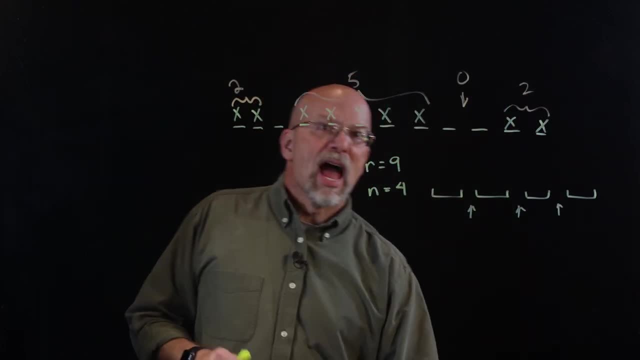 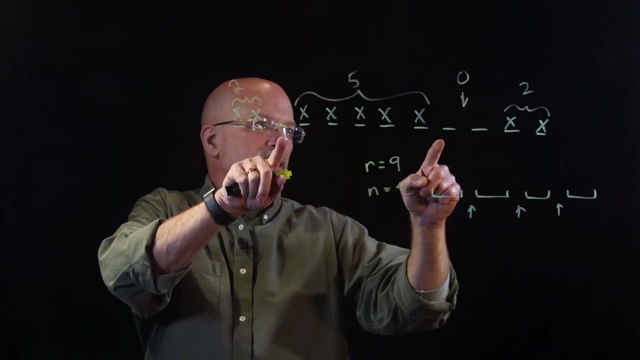 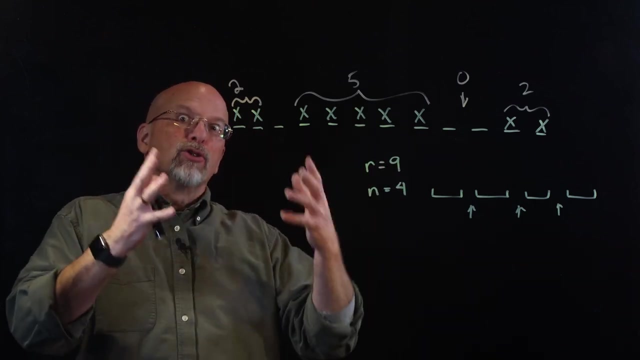 I've got two from the last element of M, and why this works is because you can come up with any combination as long as I have blank spaces in between in order to define my groups. I should you know, with the repetition, I should be able to partition or come up with a unique pattern that represents that allocation. 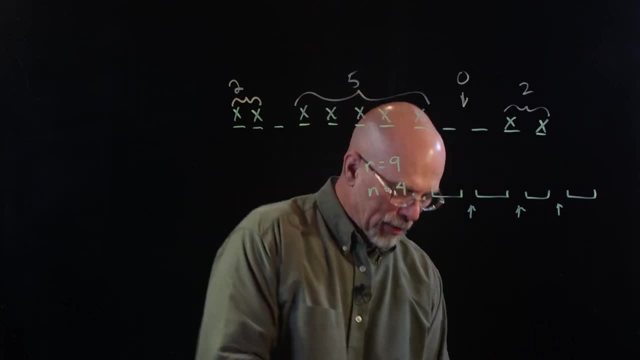 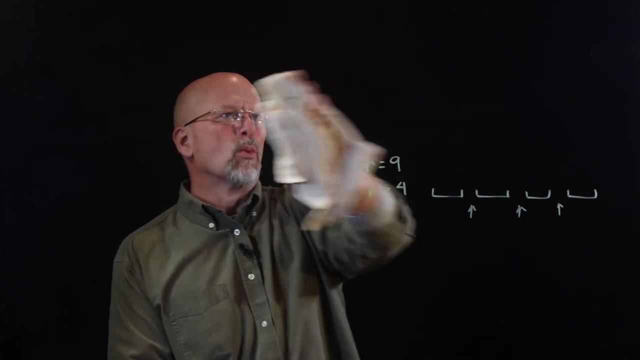 of n to 9. now, some of you may be looking at this and say, no, this is not quite right. I'm sure that there is something that won't work. well, let's, let's go ahead and come up with some numbers: 1, 2,, 3, 4,, 5, 6,, 7,, 8,, 9.. 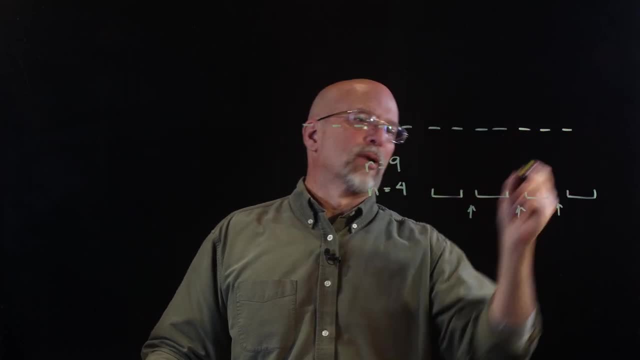 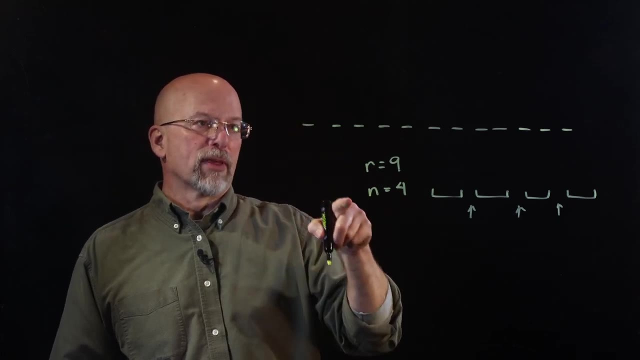 There's our 9. And then we need three spaces: 1,, 2, 3.. All right, What if the first element of n? we don't pick any, So there's none of them picked, So we actually have a space, a divider. 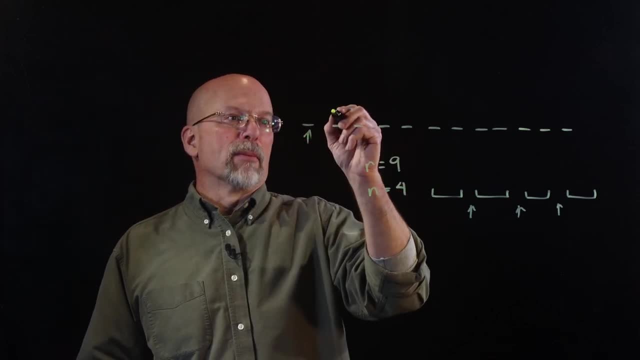 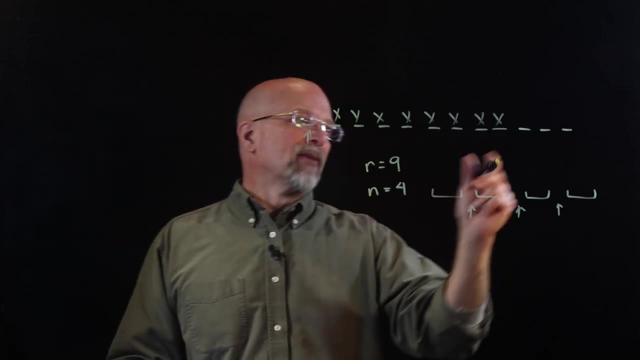 And then the next element of n. we pick eight of them: 1,, 2,, 3, 4, 5, 6, 7, 8.. All right, I've got one more to pick. I've got a space. 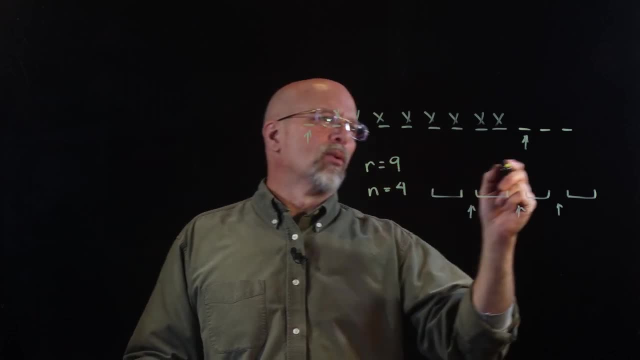 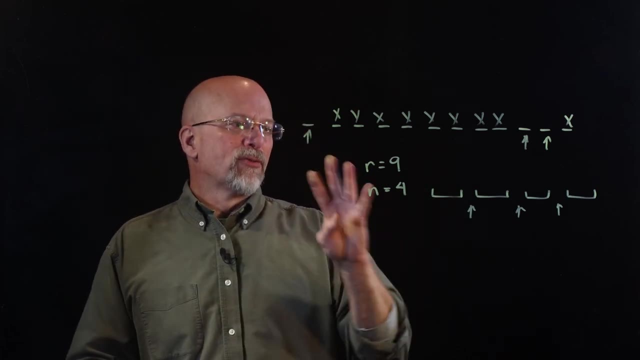 I'll pick that one. Actually, no, I won't pick that one. I'll put another space And then I'll pick the last one in the last tub. So of the four elements for n, none were picked for the first one. 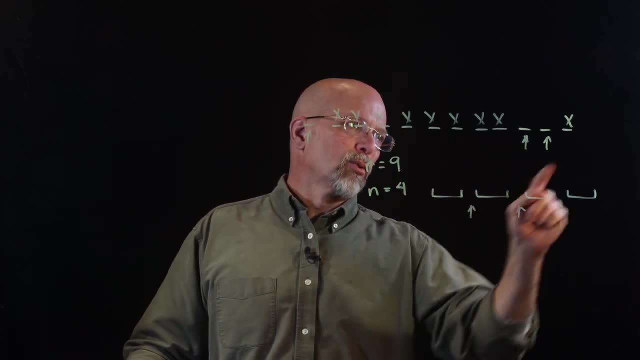 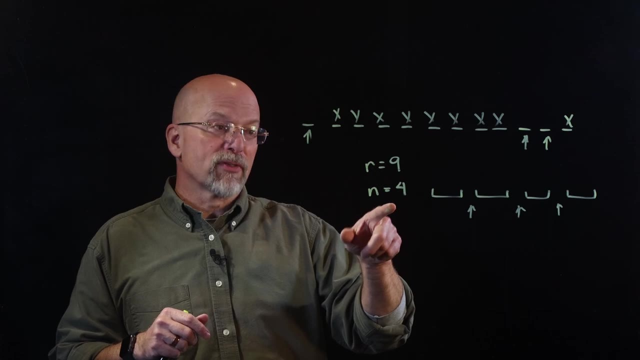 Eight were picked for the second one. None were picked for the third one. One was picked for the fourth one. All right, There is no way that you can't figure out an allocation of four elements of n to nine without leaving at least three spaces in here. 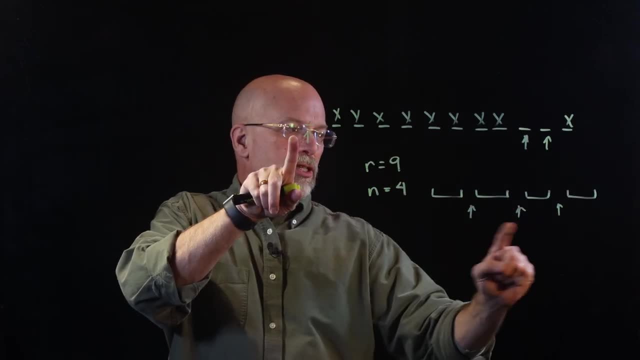 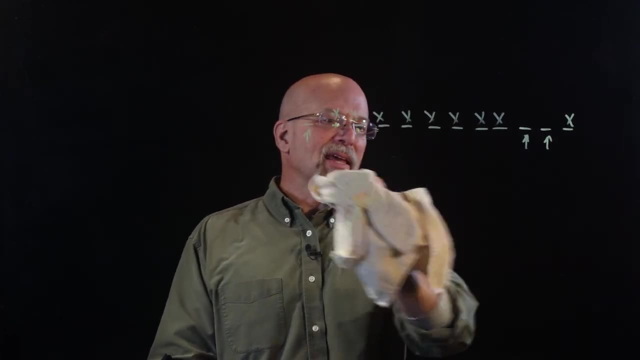 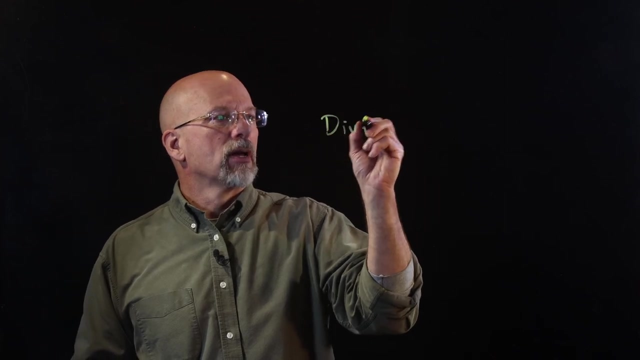 Because, remember, I have exactly three more spaces, the spaces for these three dividers, in this sequence right here. So what this is saying is: if I take, and how many spacers do I need? Well, I need or dividers, so the number of dividers equals n minus one, right. 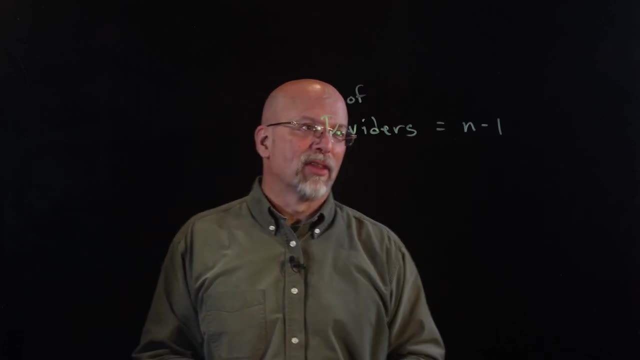 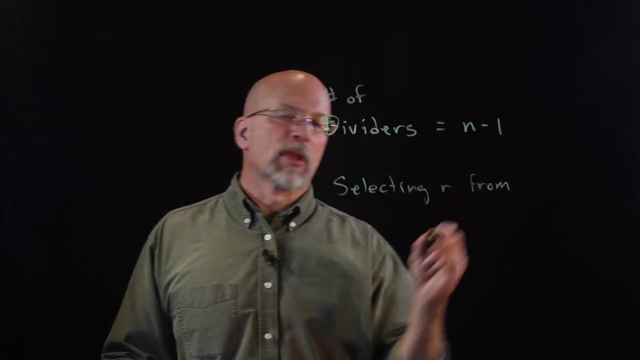 So I had those four buckets. I needed three spaces to divide them off. So I am selecting R from. well, how many slots did I have? I had R slots right, But I had to add the dividers too. 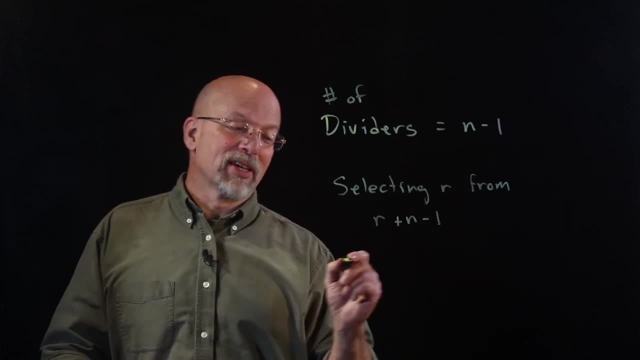 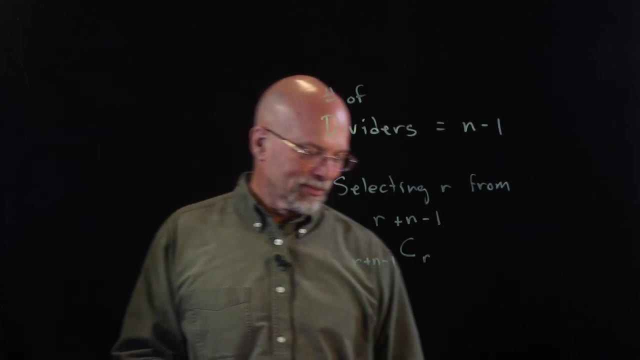 So that's plus n, minus one, And the expression for this is just simply R plus n minus one combinations. We're going to select R. Let's go ahead and apply this to some other applications. See if we're going to get this right. 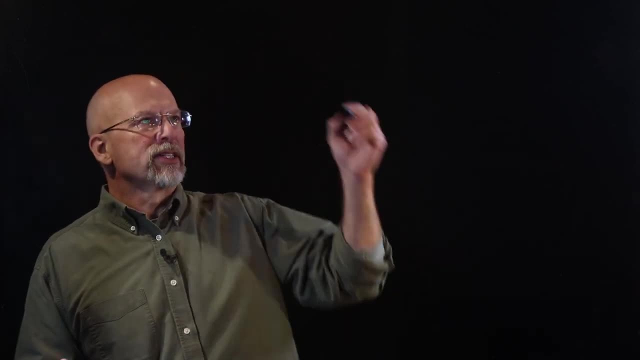 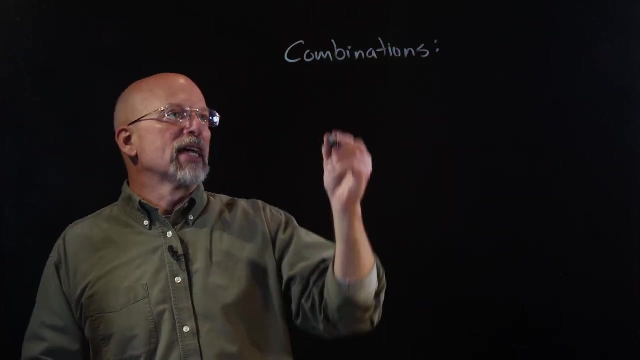 By the way, real quick, I didn't talk about this too much in the last lesson. When it comes to combinations, there are a couple of representations We could do: C, n, comma R- We've talked about this. Permutations had the same one. 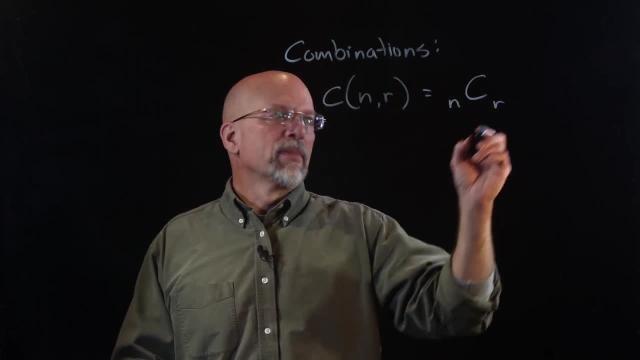 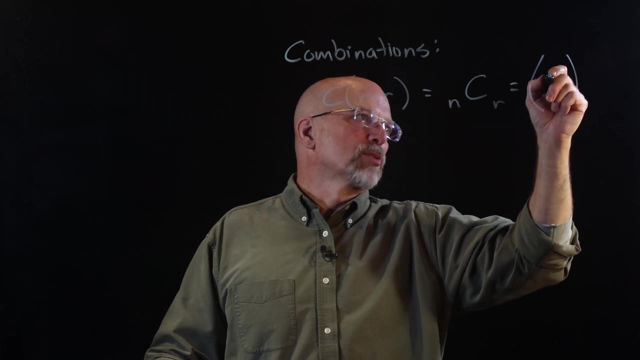 And then we also had n, C, R, And then also we could have this weird representation with these large parentheses. So you put large parentheses around an n over R. So these are the different ways. These are the ways that we can represent combinations. 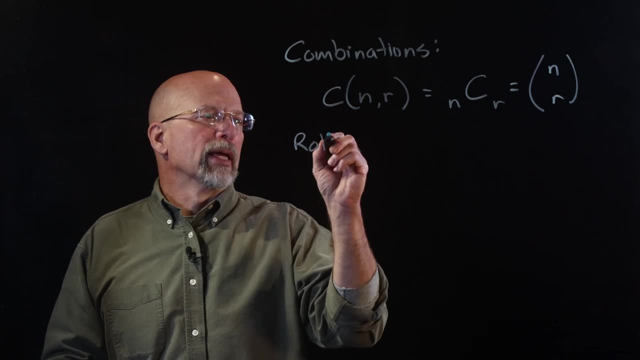 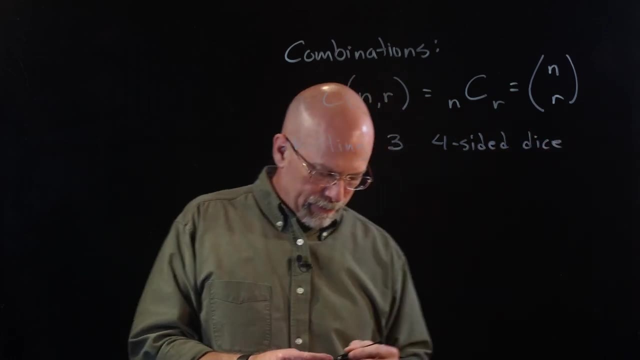 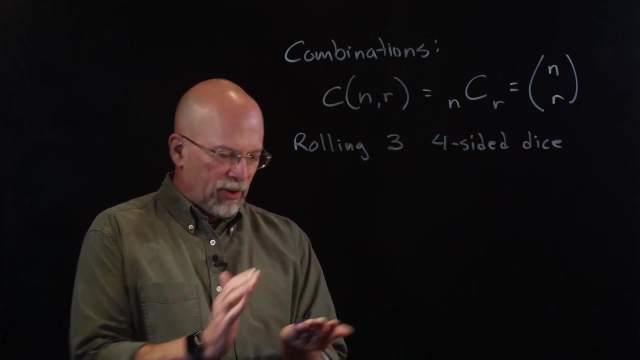 So let's say that I am rolling three four-sided dice, All right, So I've got these three dice here, These three four-sided dice, And I'm going to roll them, And what I want to figure out is how many ways could it possibly come up every time I roll it? 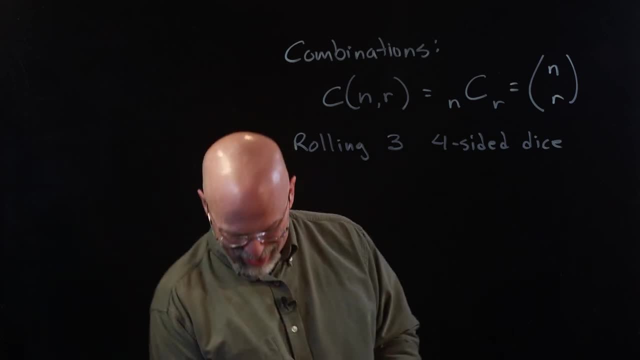 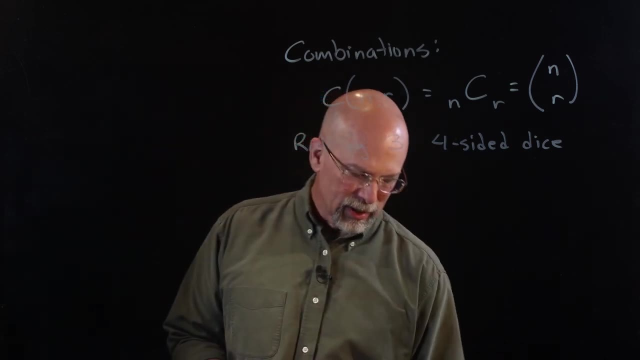 Now it's going to take me a while to get through all of them, Perhaps forever before I can come up with everything, So I'm going to use combinatorics in order to figure out what the answer is. So what is n? 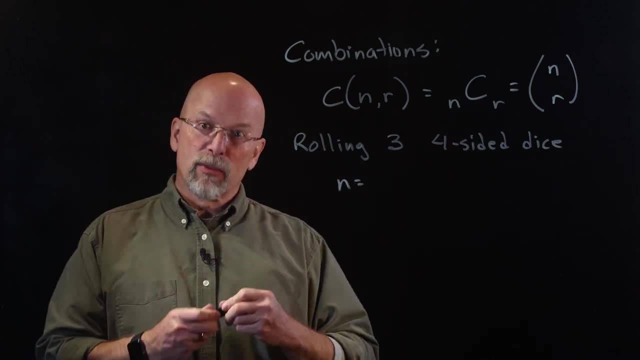 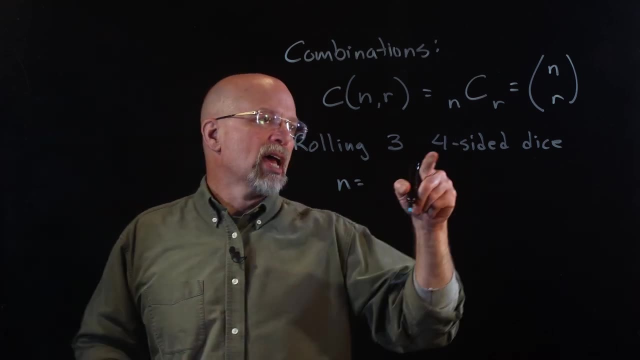 Well, remember, n is the number of elements from our set. How many different ways can we, how many different elements can we pull from a set in order to create our sequence? And in this case, it is four. right, We've got the four different numbers on our four-sided dice. 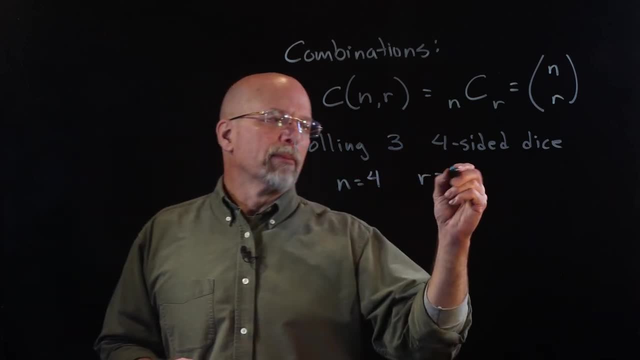 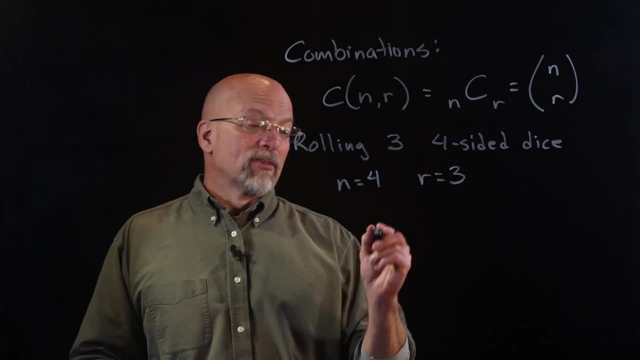 What about R? R, in this case, is equal to three, Because what we're doing is we're going to try and place these four, These four-sided values, into three slots. So what I've got are the three slots for R, right? 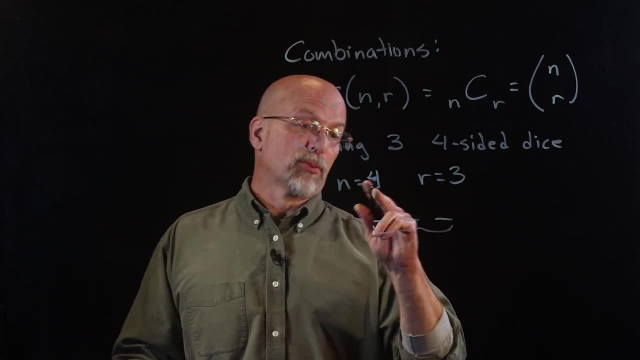 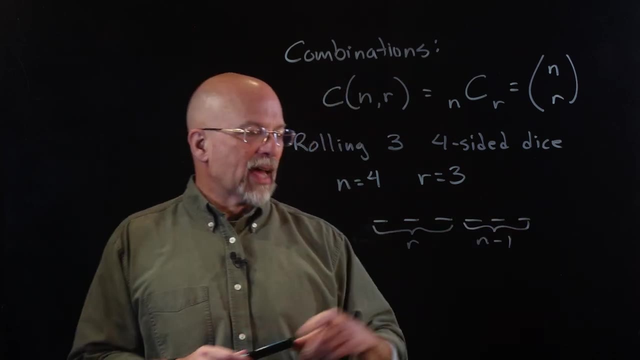 There's my R, And then I also have to have the three slots for my dividers. Remember, the number of slots that I've got is equal to n minus one. That gives me R plus n minus one- Total number of places that I can put three elements. 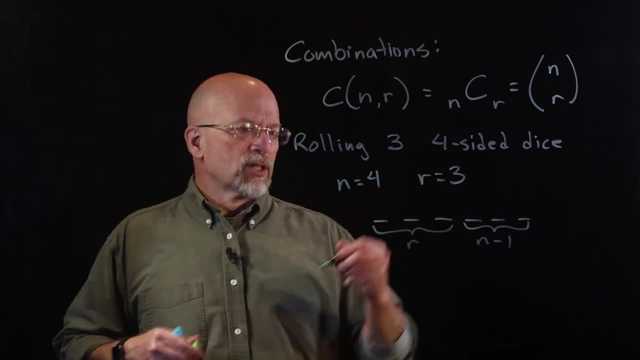 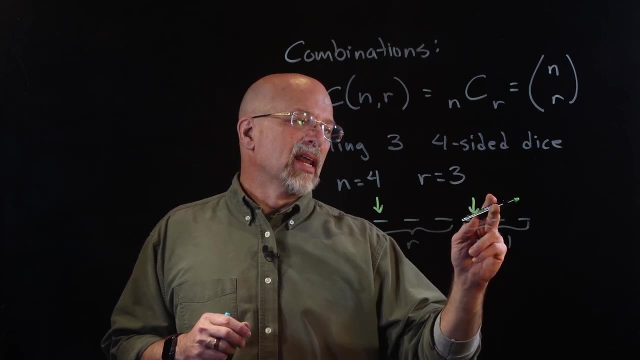 For example, let's say that I don't roll any ones, So I get my blank spot there, And then I roll two, twos. So the next one is my blank spot, And then I don't roll any threes, I roll a four. 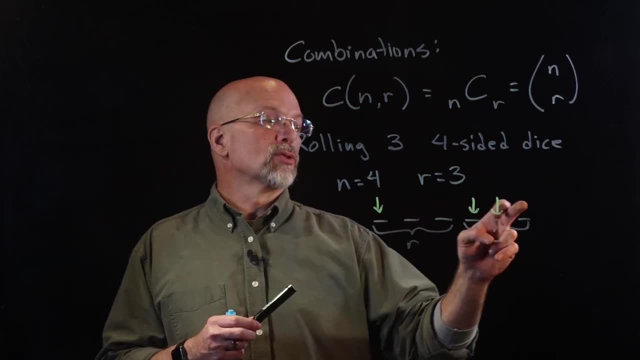 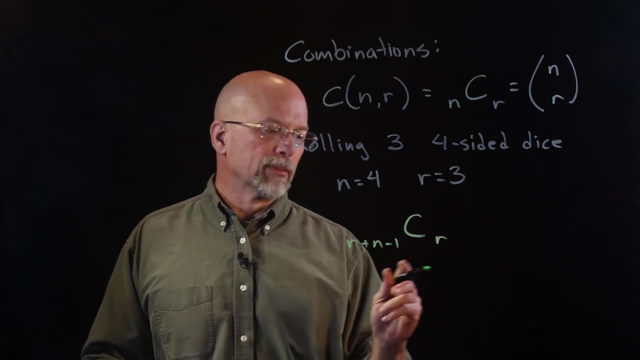 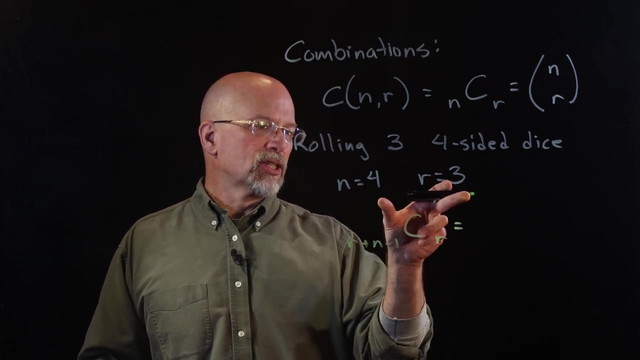 And there you go. There's the combination that would represent two twos and a four. All right, So this becomes R plus n minus one, CR. All right, So I'm pulling R out of R plus n minus one. Well, R plus n is seven minus one. 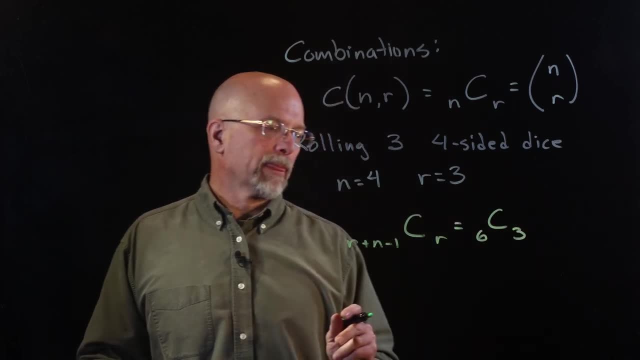 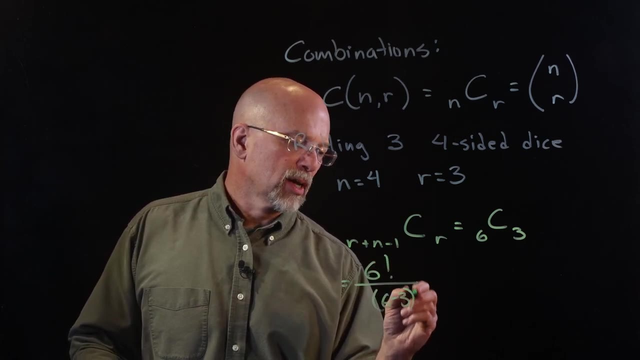 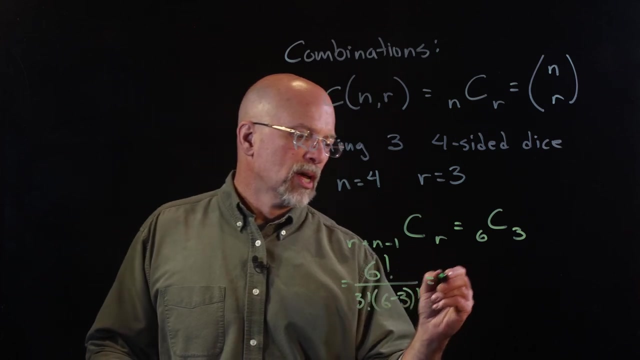 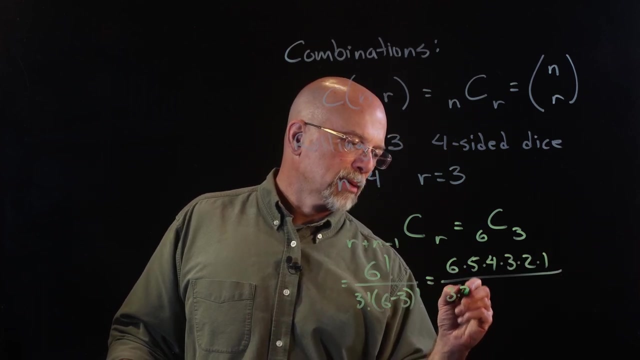 That's six Choose Three, All right. So six choose three, Six choose three is just six factorial divided by six minus three factorial right. And then we have, we pull out the orders by dividing also by three factorial. So this becomes six times five times four times three times two times one, divided by three times two times one. 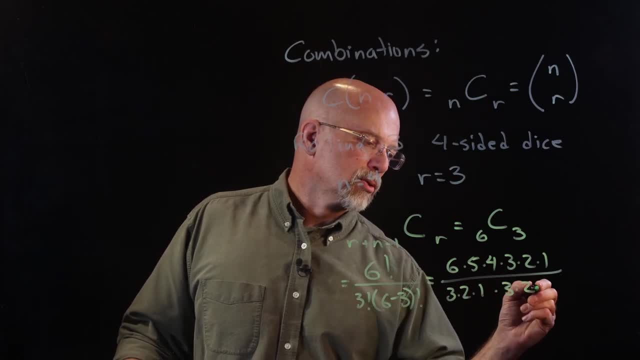 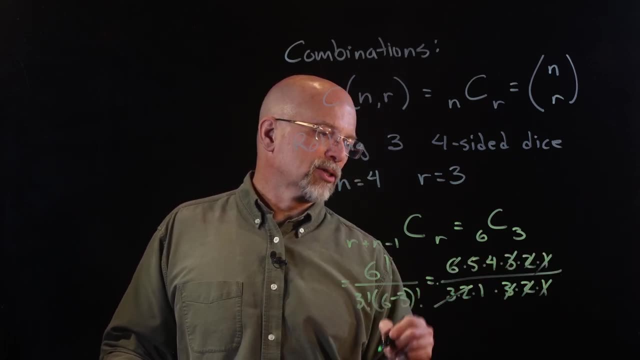 And then six minus three is also three, So it's three times two times one again, And so our three, Two, one, Those cancel out there Our three, and our two together cancel out the six, And we're left with just five times four, which is 20.. 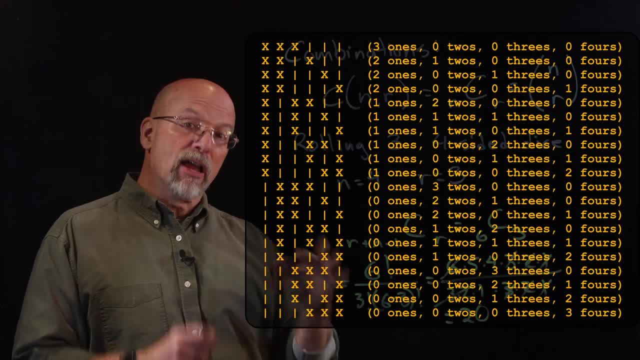 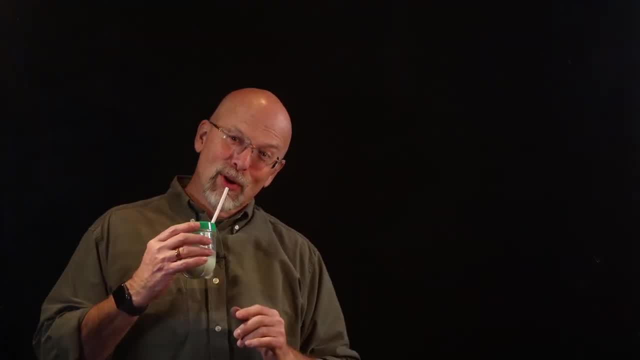 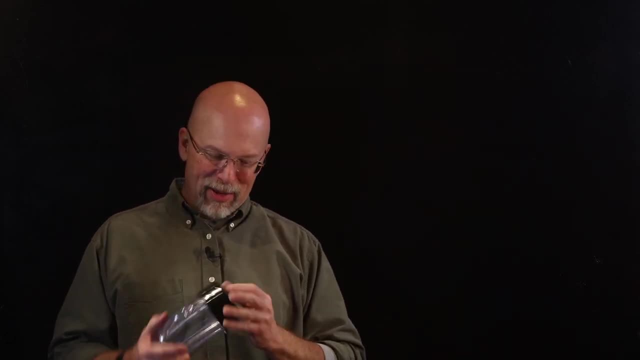 So there are 20 ways that rolling three four-sided dice could come up. So what about my smoothie? Well, I've got this little smoothie maker. I've got it doesn't hold a lot, but you put it down on a little blender thing and it blends up smoothies. 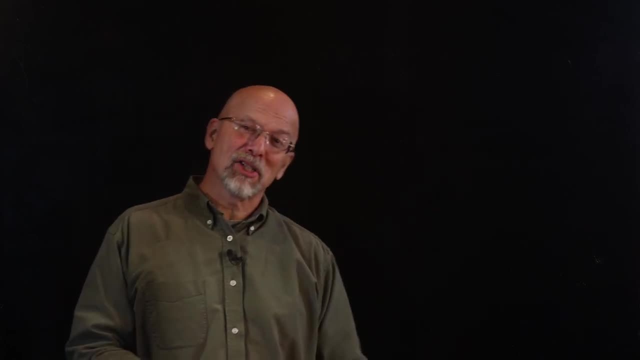 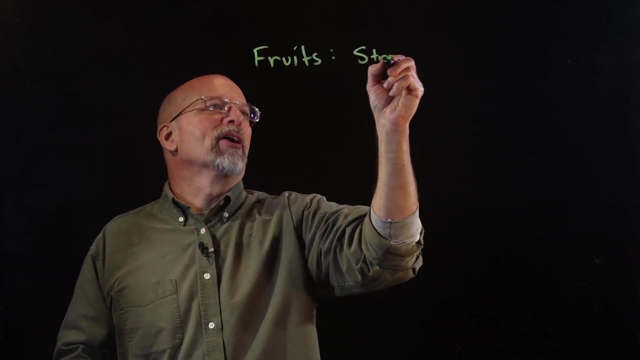 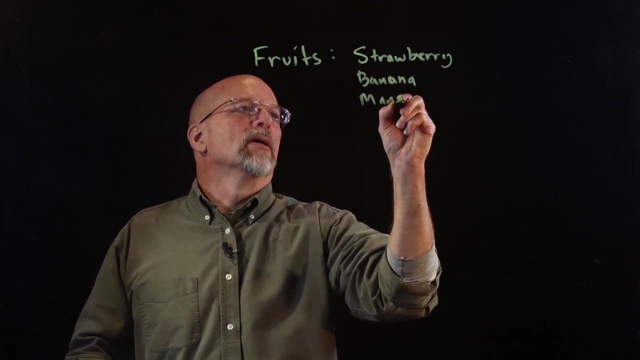 And let's say that in a year I want to open up a smoothie stand and I've got some fruits that I'd like to use in each one of my smoothies. How about strawberry? We could put banana, mango, kiwi, blueberry. 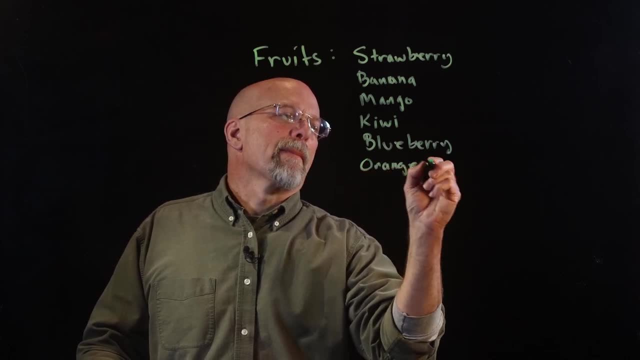 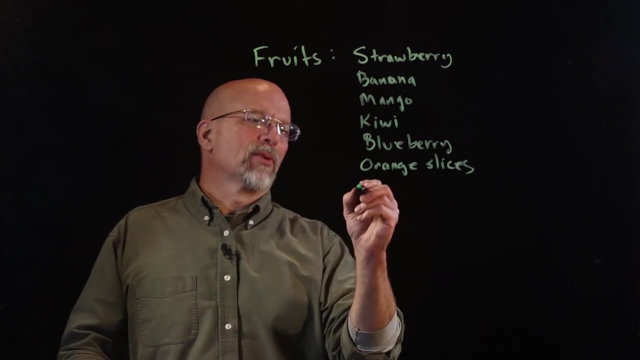 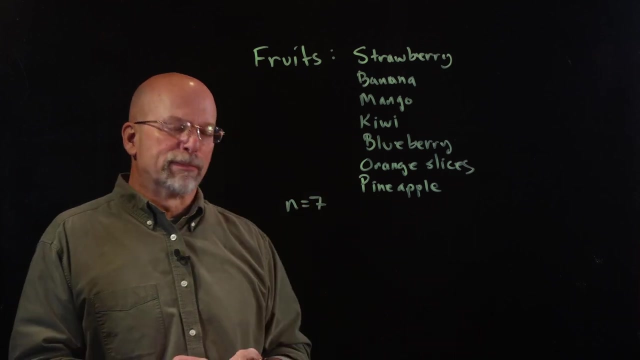 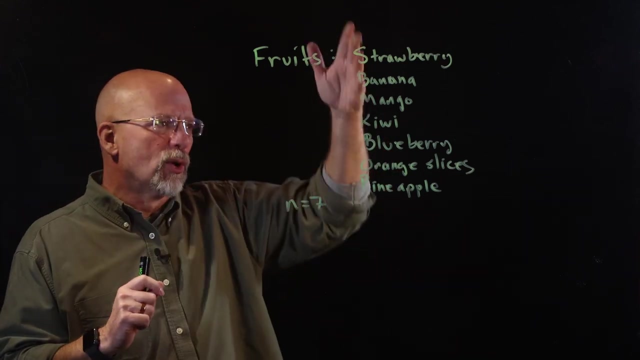 How about orange slices? What else? Um that probably looks like enough. Um, maybe we'll add pineapple to this. All right, So I've got n equal to seven And what I want to do is- I've got this plan to go through every possible combination and ratio of these guys from here until a year. 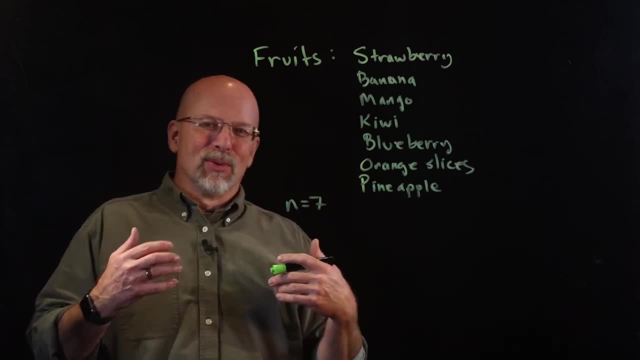 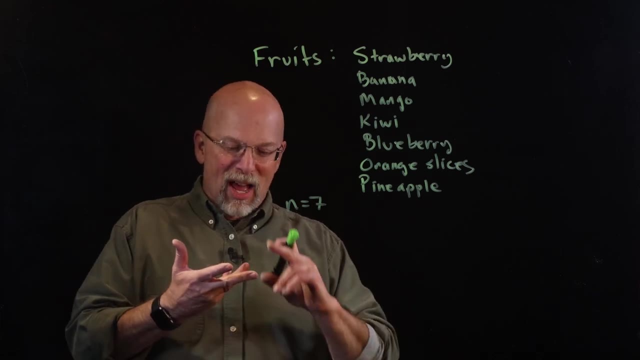 And I want to know- and I've got this ranking system, I've got do- does it? you know how's taste in terms of cost? Uh, you know, because some of the fruits cost a little bit more than others. uh, ability to hold form, you know, does does it have a good consistency? 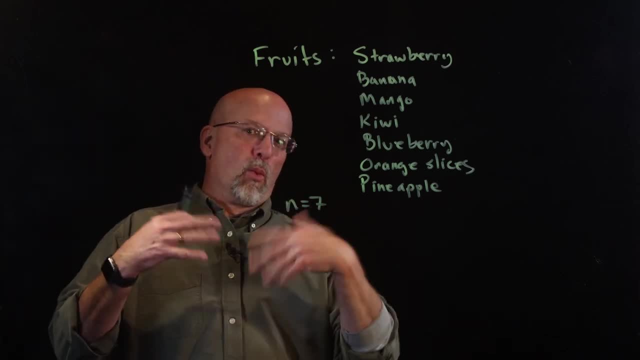 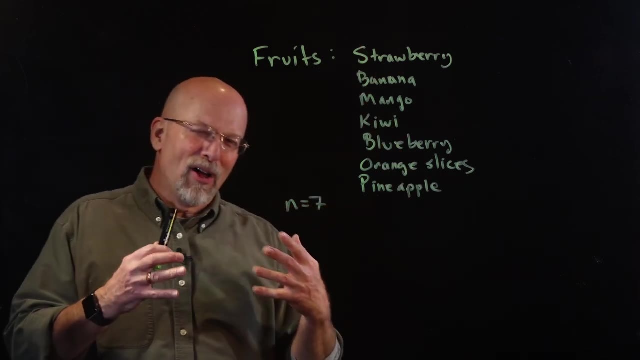 I've got this whole rating system, And so what I'd like to do is, like, once a day, have a smoothie, rank it And then, by the time a year has passed, I should have an idea of all, all of my favorite, maybe the top 10 favorite- so I can create my menu. 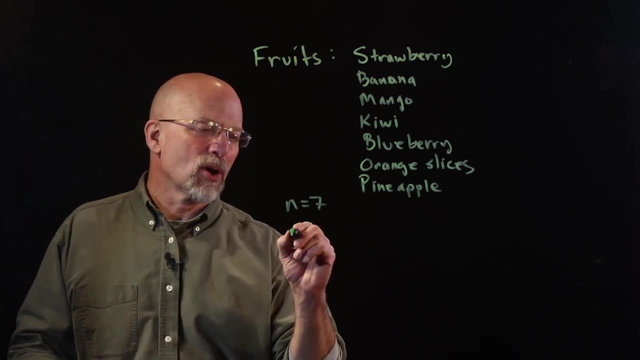 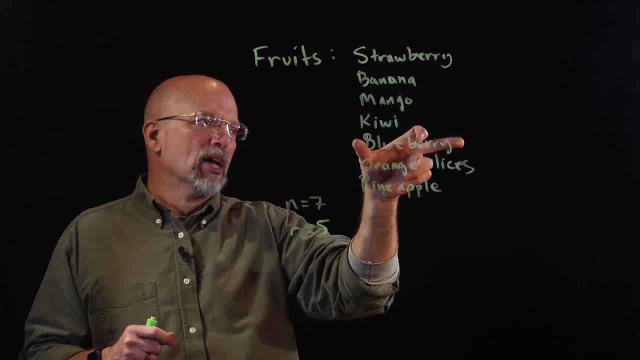 Now, my smoothie thing maker is not all that big, So I can only put a selection of five measures Of each one of these in. So I could put a measure of strawberry, two measures of blueberry, a measure of pineapple and- I excuse me- a measure of orange slices. 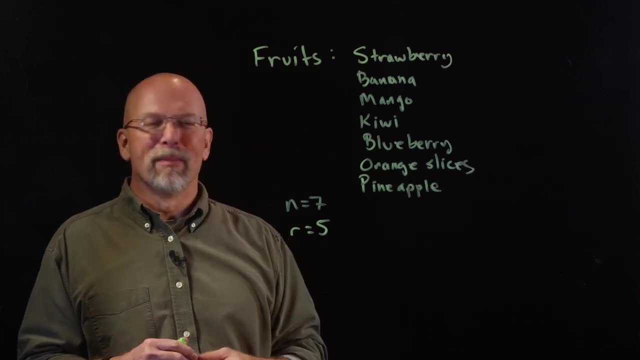 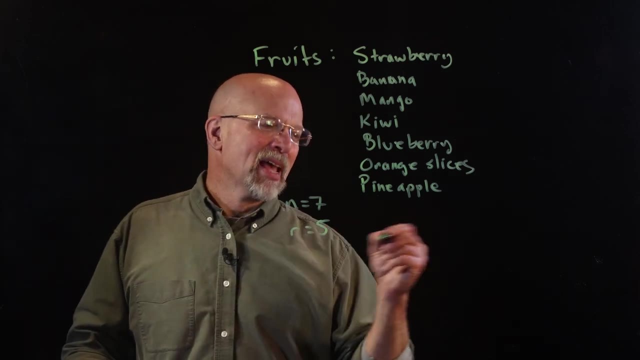 That's three, So or four and uh, I have one more measure of pineapple and I'll just go through every possible combination. How long is it going to take me to do that? Well, if I use, there's no order. 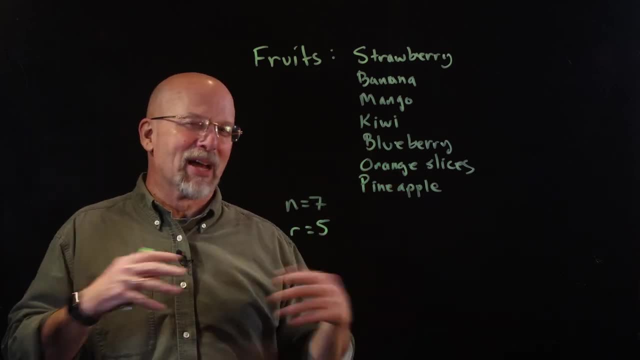 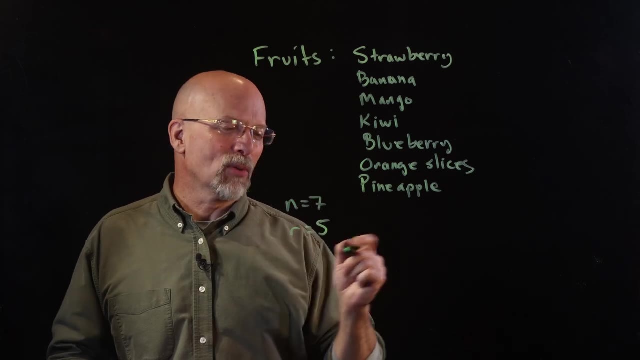 Cause once you put it in that blender, it's, it's, it's completely mixed up, no order whatsoever. So, uh, and I could have duplicates. I could make an Entire one of nothing but Kiwi. please put in the comment section. 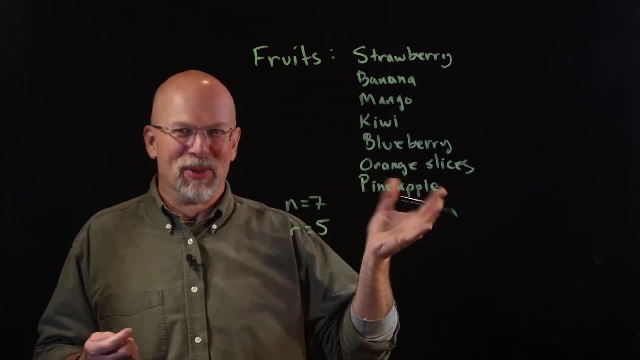 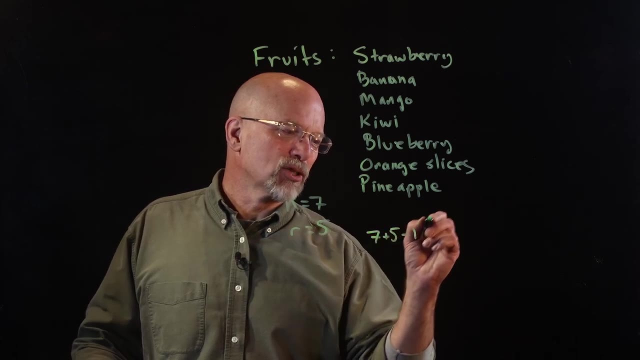 If you think these are a bad selection, I have no idea. I don't drink smoothies, to be honest with you. Anyway, what we've got is, uh, seven plus five minus one. choose five using our system. Okay Now, so this is seven plus five. 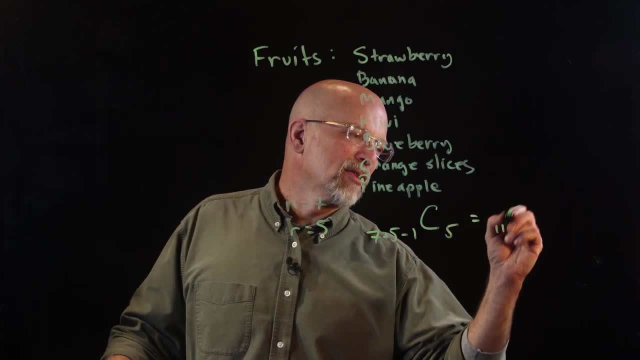 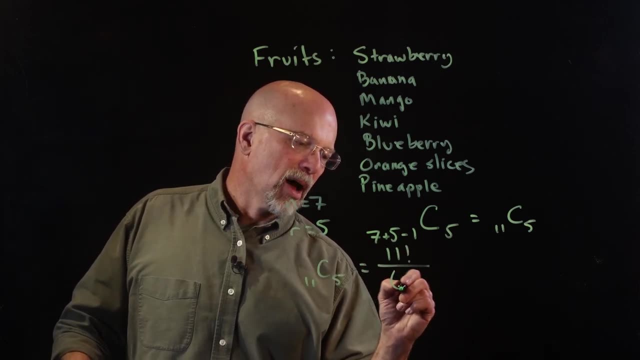 That's a 12 minus one, That's 11.. So this is 11 shoes Five. 11 shoes Five is equal to 11.. Fact Oriole divided by well, we're going to start out: 11 minus five. factorial. 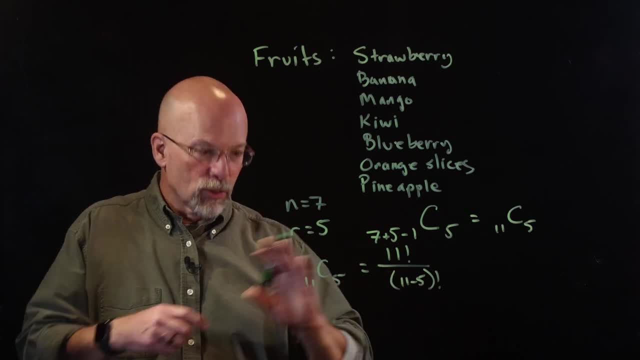 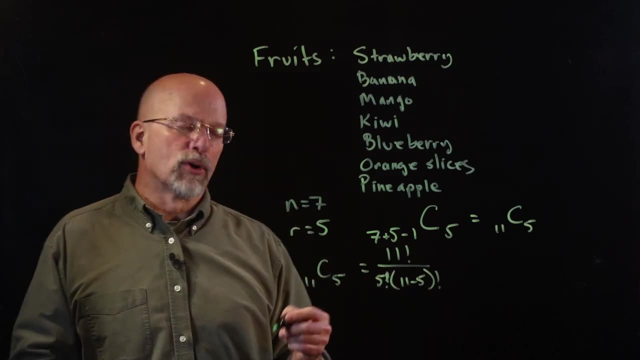 And that is that is going to um, take out the ones that we don't pick for that particular run, And then we're also going to have five fat, divide by five factorial, in order to pull out any of the- uh, any of the order, whenever we do finally select five. 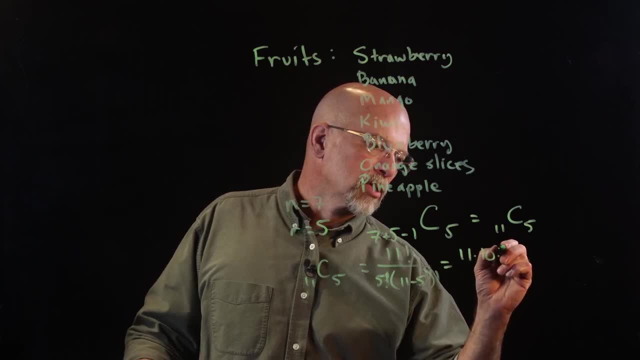 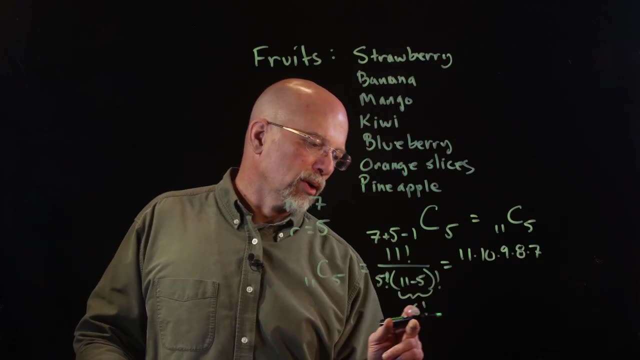 And so this is going to give me 11 times 10 times nine times eight times Seven. Um, this guy right here is equal to six factorial. So when you divide six factorial into 11 factorial, you're left with 11 times 10 times nine times eight times seven. 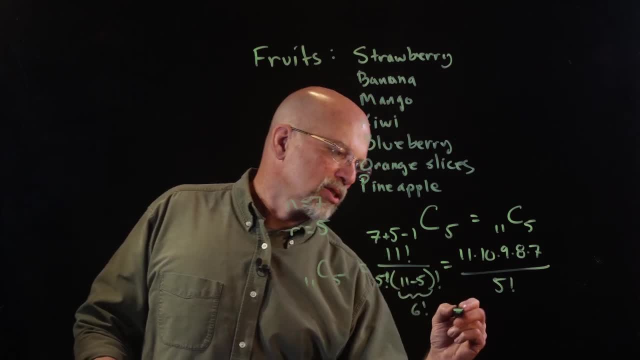 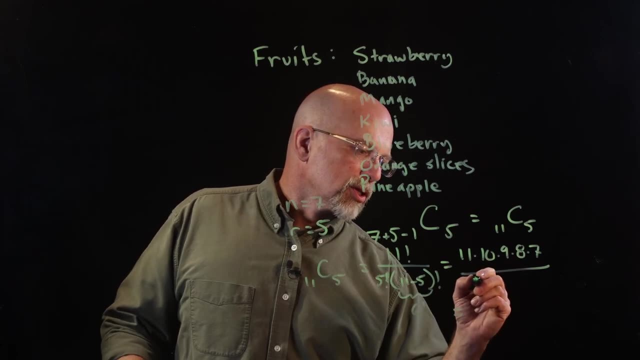 And then we're going to divide by five factorial, And so this is going to give us, well, actually, five we can take out of what do we have? Five factorial. Five factorial is just equal to five times four times three times, two times one. 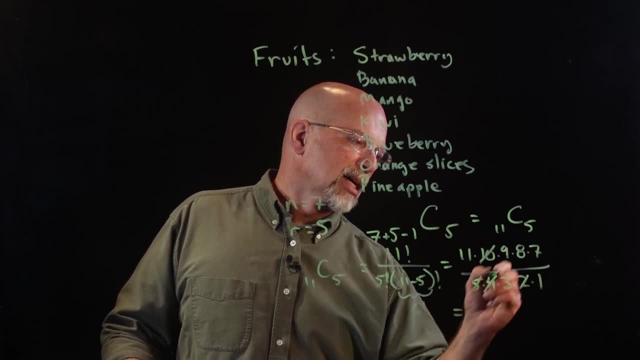 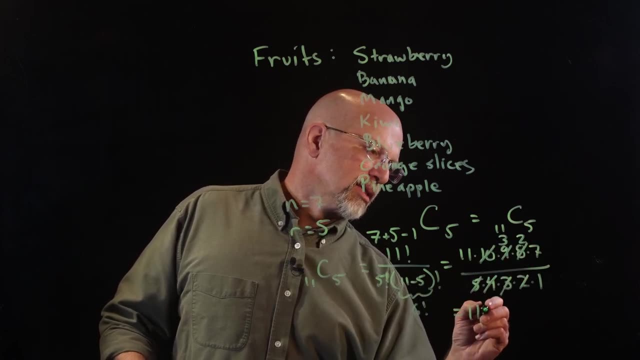 Let's see: the five and the two can cancel out the 10.. I can take a four out of eight, I can get two. I can take a three out of nine and get three, And so really what I've got is 11 times three times two times seven, which is equal to 462.. 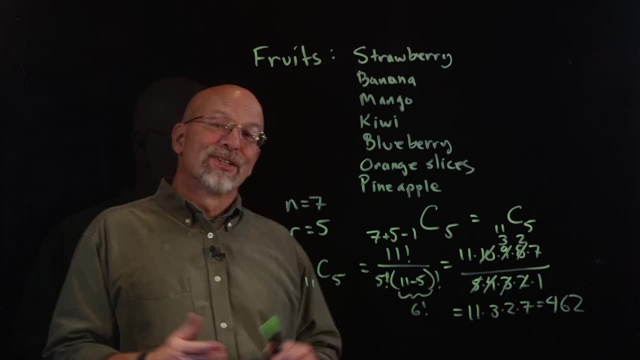 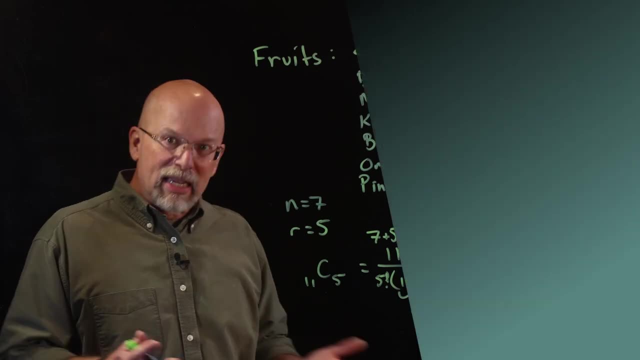 Wow, I better get started drinking soon. huh, So there you have it. enumerating and counting the possibilities by hand, especially for large values of N or R, can be darn near impossible, but we have all these expressions. We've got N to the R, we've got NPR.